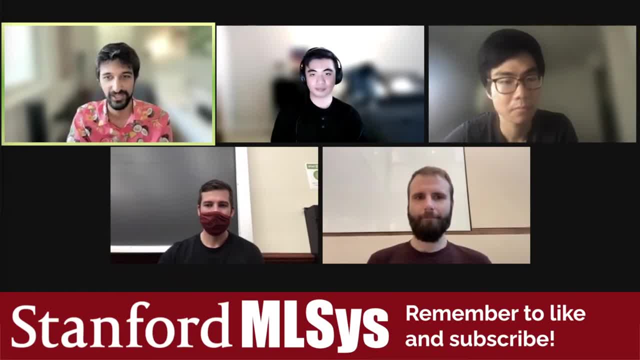 by a 30-minute podcast-style discussion where you in the YouTube live chat can post questions and we'll get those questions across to Albert. You can keep posting those questions during his talk and we'll aggregate them and get those across. A little bit about the talk today, so Albert's 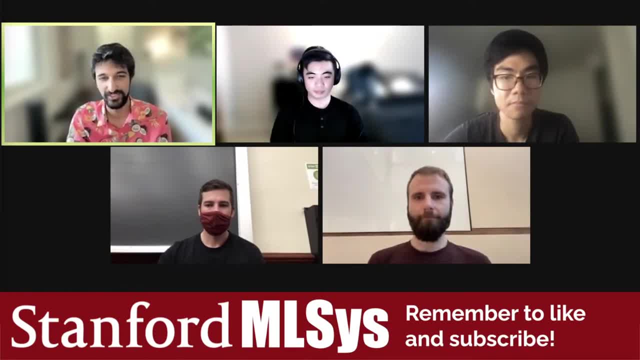 going to be talking to us about modeling long sequences with structured state spaces and he's going to describe a new model that he's built. He is a PhD student in Stanford, the Stanford CS department, advised by Chris Ray, and is interested in structured linear algebra and the theoretical 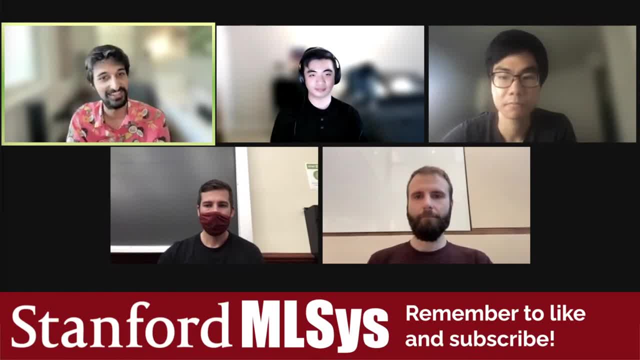 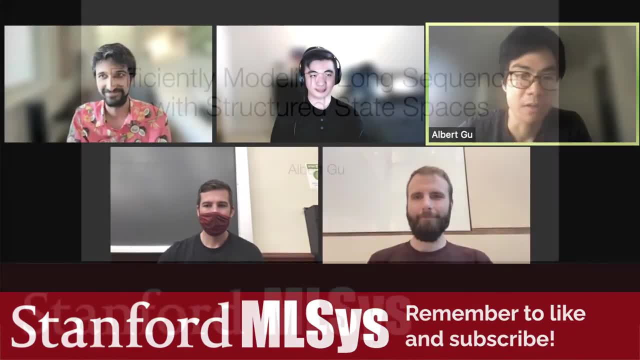 properties of sequence models. He's also on the job market, in case there are any folks listening, so he's going to be talking a little bit about the talk today. Take it away, Albert. Thanks for the introduction, Karan. All right, so, as Karan said, in this talk I'll be introducing a. 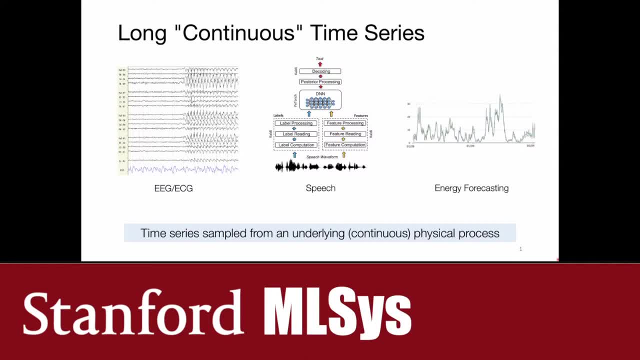 new sequence model To set the stage. first, let me just talk about the types of problems that we hope to solve. So we're going to address long and implicitly continuous sequences as our main motivation, and I'm just going to call these continuous time series. To give some examples, 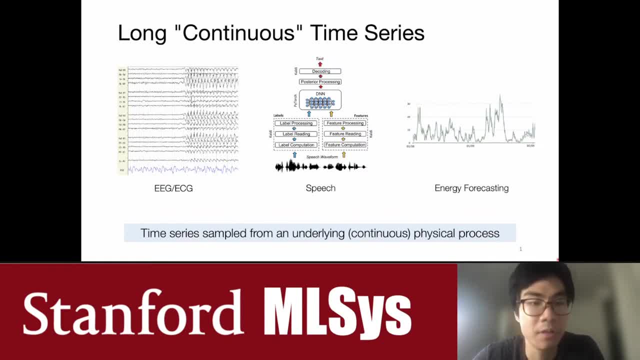 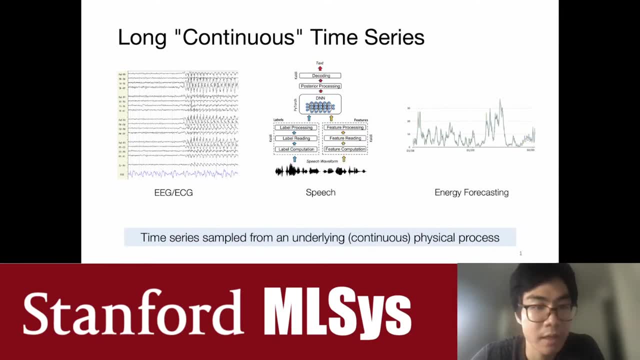 on this slide. here are some examples of typical time-series data of this nature. On the left is medical time series such as EEG or ECG signals, in the middle is a typical speech waveform and on the right are energy forecasting signals. So, in general, continuous time series are defined by sequence data that's sampled from an. 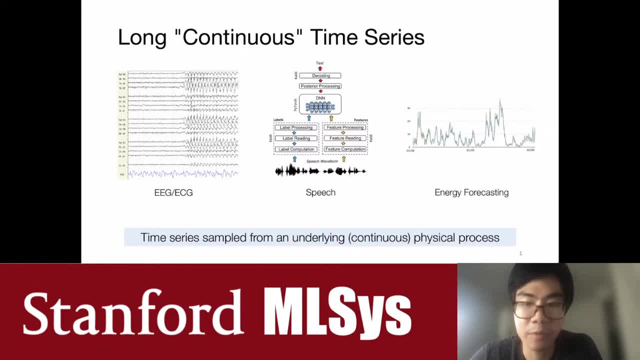 underlying continuous signal. This type of data is something that people don't usually think about when talking about sequence models, but it's a very challenging type of data with unique characteristics. So, for example, speech data is typically sampled at 16 000 hertz or even higher, which means that for clips of just 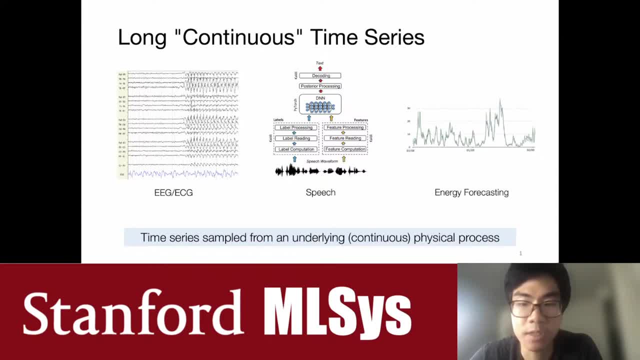 one or a few seconds. the sequences are tens of thousands of samples long, which is already much longer than what deep learning models can typically deal with. so, unlike other ml fields, like vision, where end-to-end deep learning models perform well- in speech, for example- typically you need to rely on substantial feature engineering and complicated pipelines. so in this talk we're 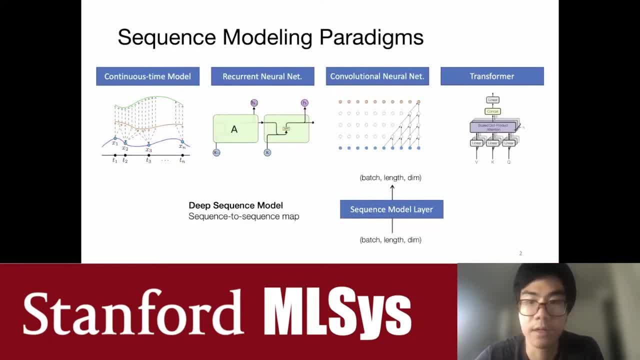 going to try to address these with um using generic deep sequence models and for the purposes of this talk, i'm defining a sequence model as just a sequence, the sequence map composed of primitive layers, um where, concretely, each layer should operate on a sequence of inputs. 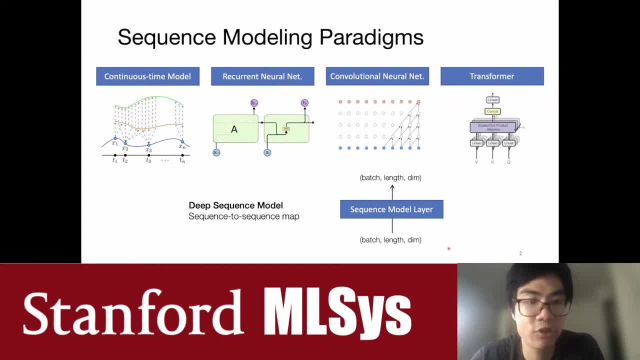 that is a sequence with a hidden dimension and output something of the same shape, and give some examples um up top are some classical families of deep learning models that satisfy this interface. these include continuous time models, recurrent neural networks, convolutional neural networks and transformers. these families all have um different strengths and weaknesses. 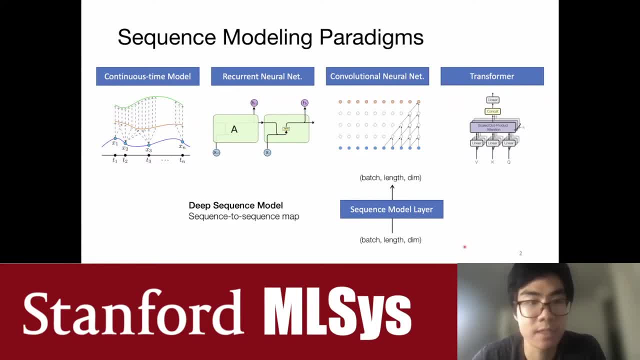 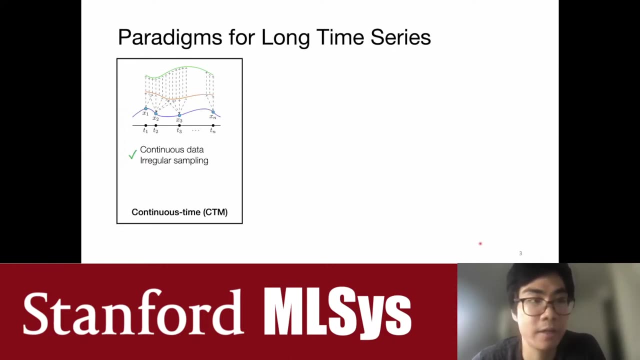 when it comes to modeling sequences, but for continuous time series, like the motivating examples. these first three are more conventional and i'm going to focus on them first for now. so in a little more detail. we define continuous time models as models that directly try to model the underlying continuous process of data. 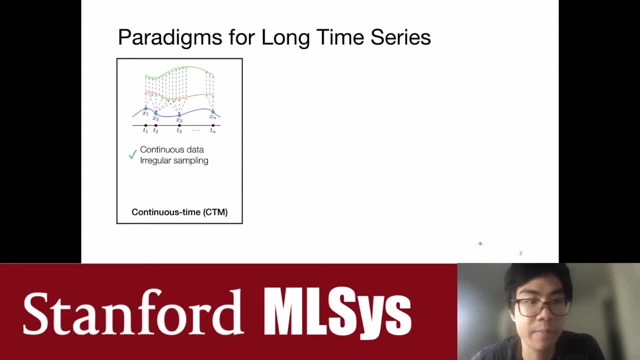 um. this allows them to capture the inductive bias of this type of data better and perhaps automatically do things like handle missing data and other applications. recurrent neural networks, or rnns, are a natural stateful model where they summarize information they've seen to a hidden state and so they're better in certain settings. in stateful settings, like reinforcement learning. 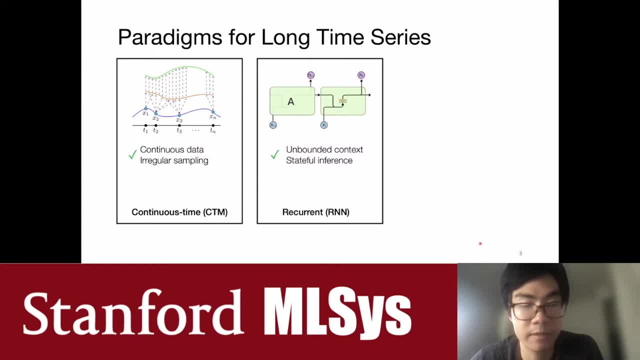 and they can also perform certain autoregressive tasks more efficiently. and convolutional neural networks, or cnn's, are easily parallelized, so they're much more flexible, so they scale much better and are much easier to train than the others. so every model has clear strengths but also has clear weaknesses. so, for example, continuous time. 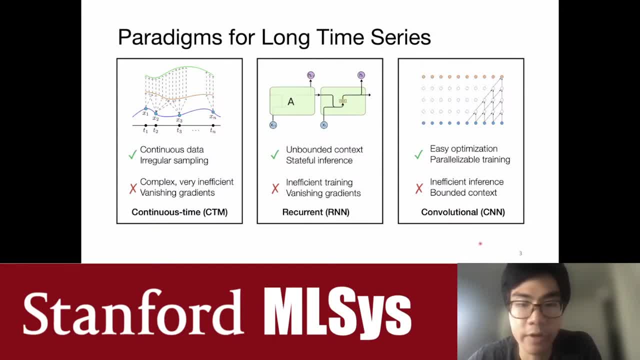 models and rnns are both slow and they suffer from what's called the vanishing gradients problem because of because they're inherently sequential. on the other hand, cnn's don't have this problem because they're kind of more global and parallel, but they do have inherently bounded context, which 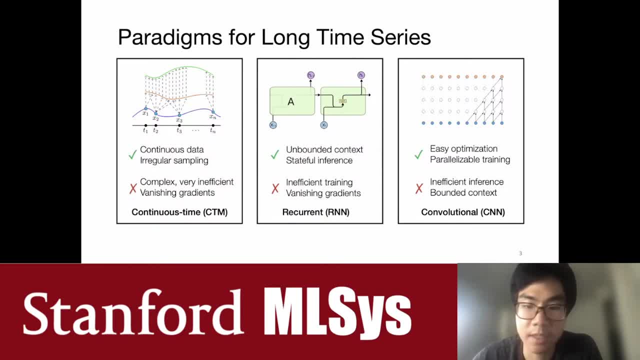 makes them um more visible to your karena with over time- and that's one of the underlying strength of this model- and then actually having these fallback within your region, it was somewhat of vens creasing propia luciana rodzley's model. this is the observator involved, girl. 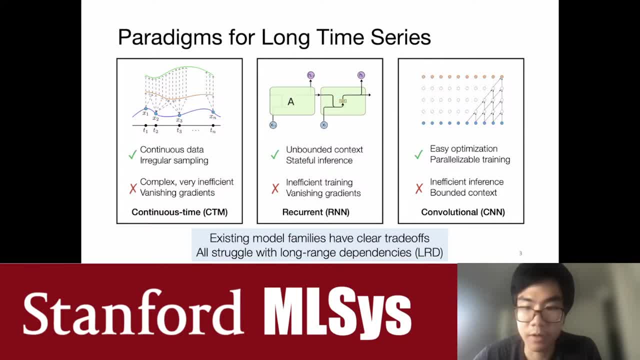 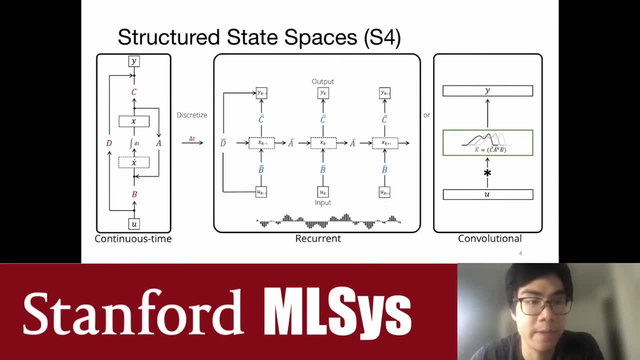 that replaced her in mind. view of by the vanishing trajectory rn is really interesting because the rnns has a similar structure to the rnns of thelength and also frogman developed with that floor. so again, on this example we they lose for computed lasik in our DevelopEC model. 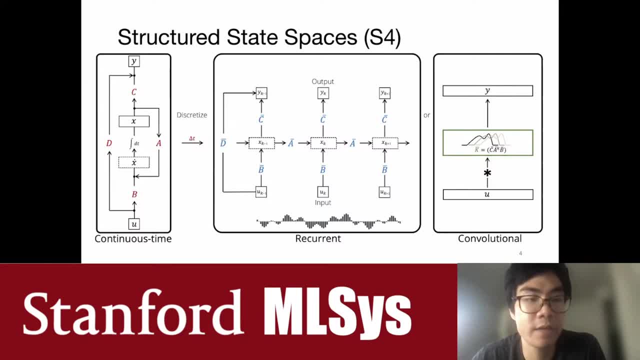 So the high level is that this model is going to have three different representations that can be switched back and forth between each other, and each representation gives it the benefits of one of those three paradigms: continuous time, recurrent or convolutional. 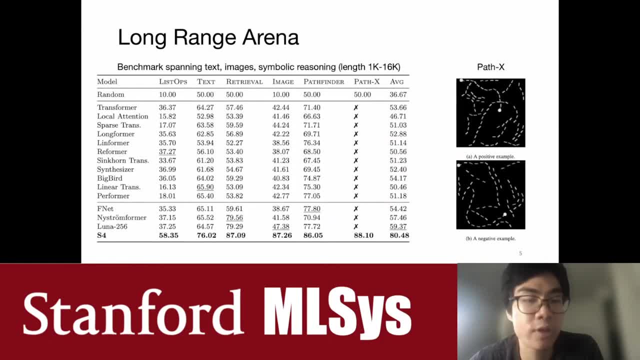 All right. so as a little preview of the results, here is a recent benchmark for long-range sequence modeling. It consists of six tasks across many different types of data that span from 1,000 to 16,000 length sequences And, for context, usually in sequence modeling things that are even 1,000 or even like a few hundred steps is often considered long context. 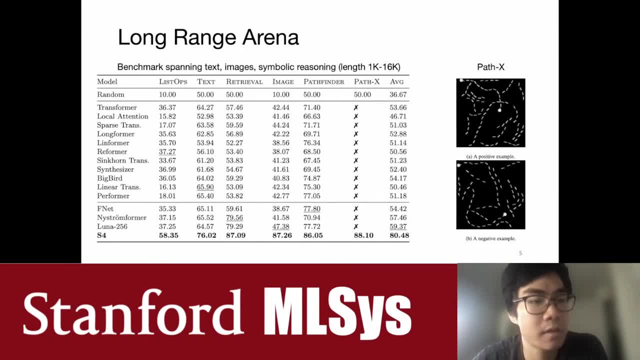 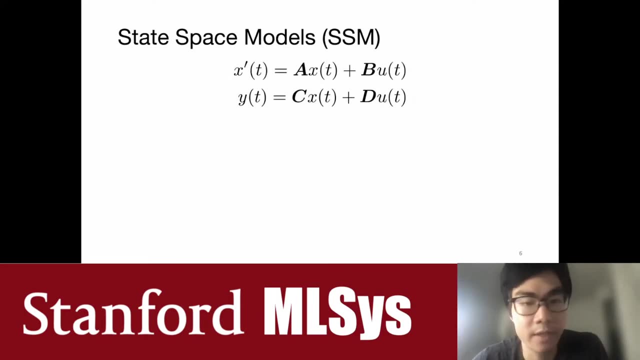 So this is extremely long context and our new model does really well in this benchmark and outperforms every baseline that we're aware of by a substantial margin. Okay so? So first I will introduce the model and walk through a bit of the mechanical details. 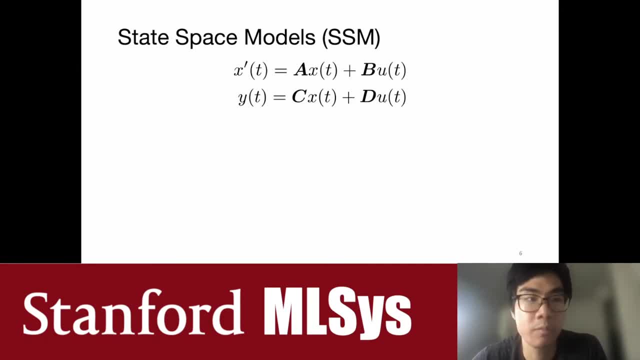 So the model is based on the state-space model, which is a well-known model in many scientific and engineering fields. It's defined by just these two equations. So the way we think about it is that we think of these two equations as defining a parameterized function-to-function map. 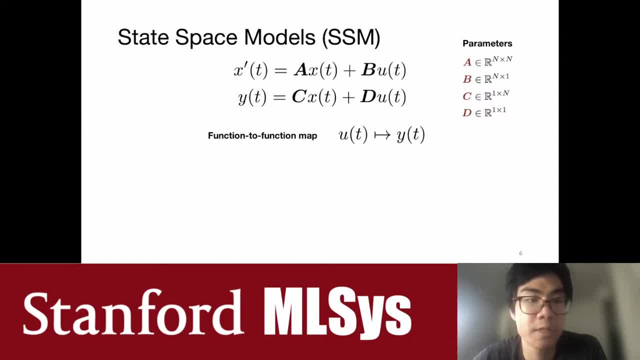 And throughout this talk I'll use the same notation- Where U denotes an input sequence or function and Y denotes the output sequence or function of our sequence model layer. So here we think of the state-space as a map from. it's a parameterized map using parameters A, B, C, D and it maps some input function U to an output function Y. 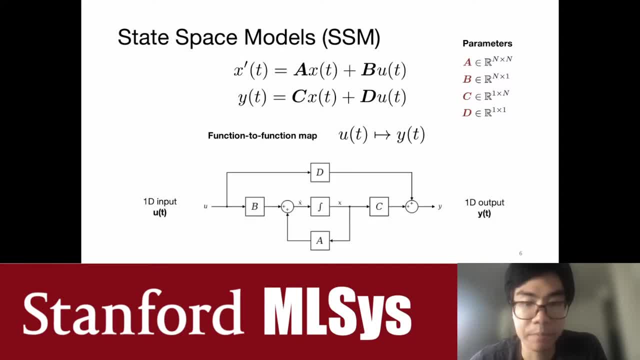 It's sometimes drawn with this sort of control diagram And going in a little more detail. basically, the first equation here can be thought of as taking your input, U, and expanding the dimension into a latent state X, following a simple linear ODE. 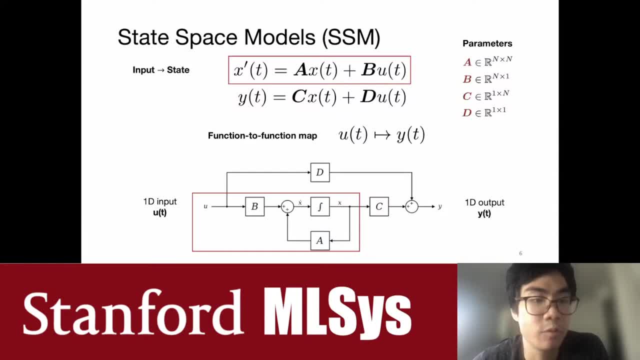 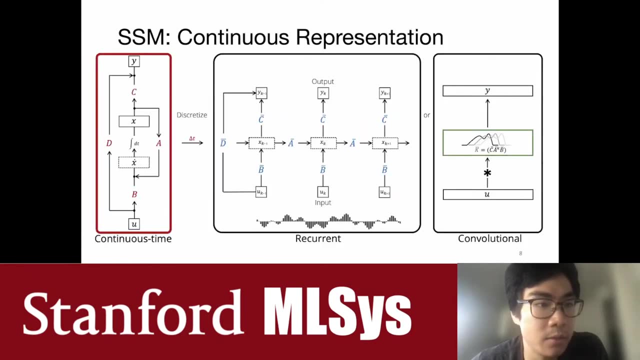 In the control diagram you view it as passing the input through some sort of feedback loop, And then this hidden state X then gets projected out to an output that has the same dimension as the input. So turning the diagram on the side gives the input a little bit more space. 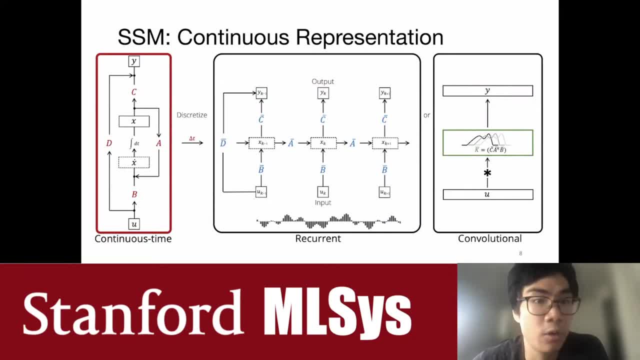 This can be seen on the left part of this diagram. So, at its core, we will be parameterizing our model using these parameters- A, B, C and D, And this is implicitly a continuous-time model that defines a function-to-function map. 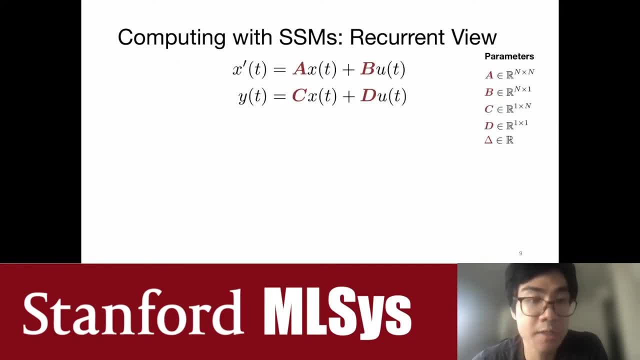 Now to work on sequences instead of functions. we will need to convert this from continuous-time to discrete-time And basically the way this works is that there is a. there are some certain well-studied formulas or transformations that can take your continuous time parameters. 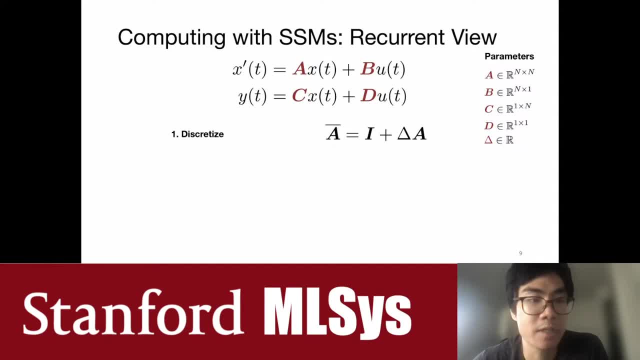 a, b, c, d- into discrete parameters: a bar, b bar, c bar, d bar. They're basically just simple formulas of the original parameters And then, given these discrete parameters- a bar, b bar, c bar, d bar- which I'll be denoting with blue in general, your continuous time model gets. 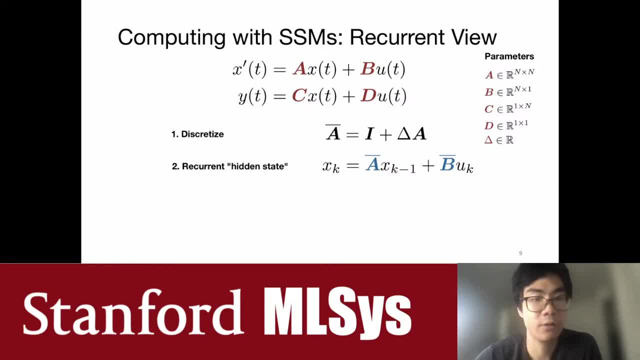 transformed from a differential equation into a recurrence. So now here we still have an input u, the input is still u and the state is still x, but instead of a differential equation it follows a very simple linear recurrence that defines this hidden state And then the hidden state. 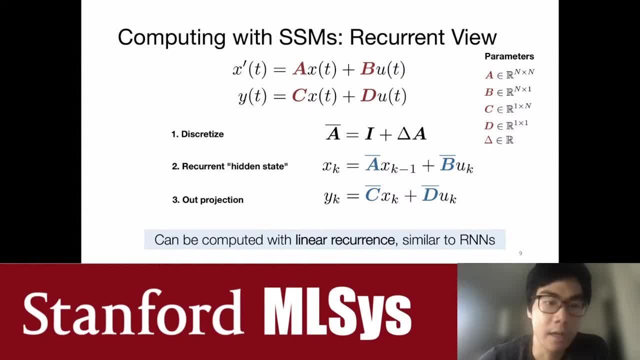 gets projected back out to an output y. So, basically, the original state-space model can get transformed into this linear recurrence that has very similar form but using a slightly different representation- a bar, b bar, c bar and d bar- And so the upshot is that the discrete version of the state-space model is, in fact, a simple 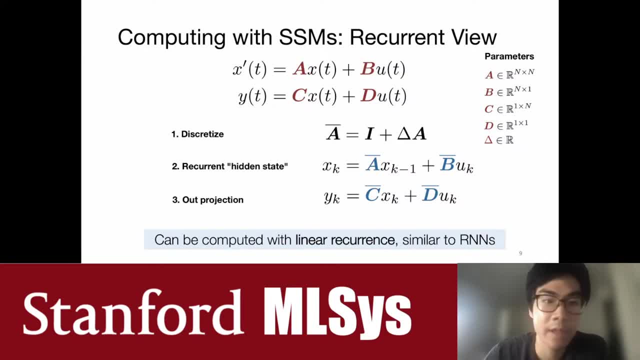 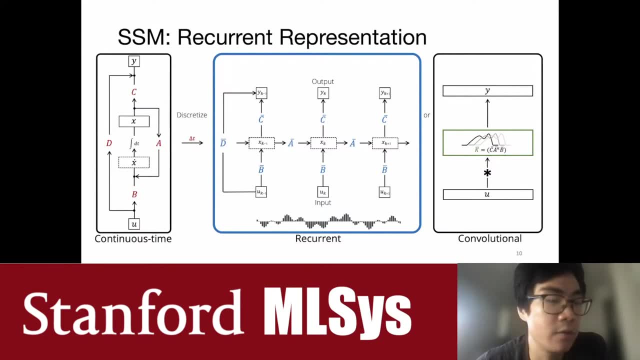 linear recurrence or a linear RNN, And in the diagram, basically what you can view this: you can take your original continuous time feedback loop and unroll it as a discrete recurrence in discrete time And it looks exactly like this. So you can see that the 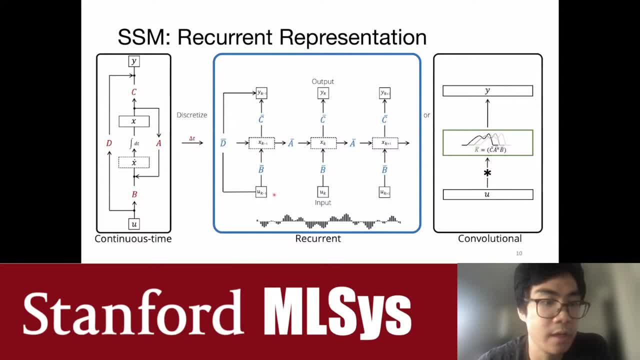 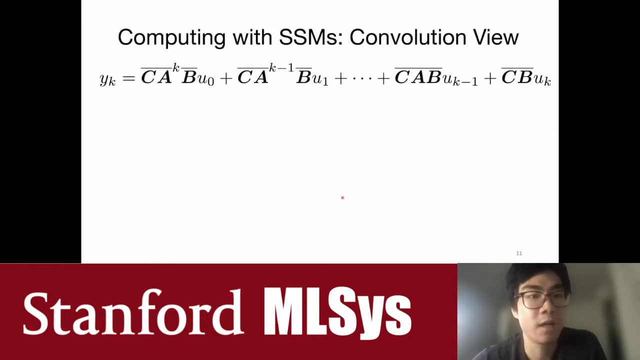 input is like an RNN, So you feed your inputs u in one at a time, and for each input you update your hidden state and then project it out to an output. Now the final view is the convolutional view, And the main idea here is that the because it's- 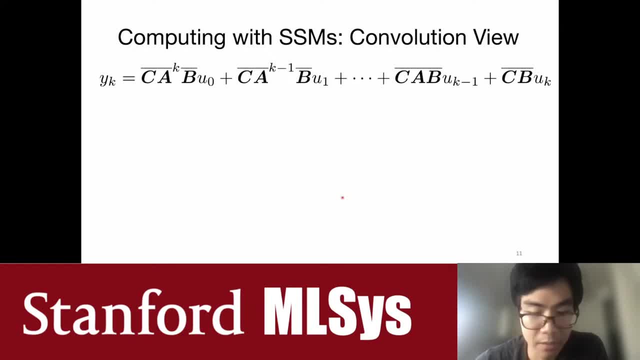 a simple linear recurrence. you can actually unroll it in closed form. So here, remember again, inputs are sequence u and the outputs are sequence y. And it turns out you can just unroll this recurrence by hand and derive a closed formula for the output in terms of the input. 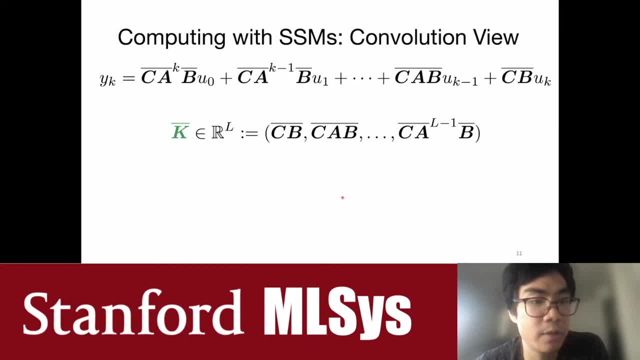 And then by collecting certain coefficients into a representation that we call k-bar, then it turns out that the entire output vector y is a simple convolution of the input vector u, And so this is actually the most important representation, and we'll see why later. 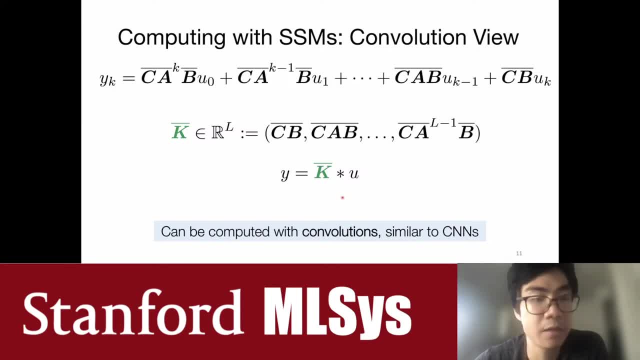 But this is the way we usually train the model And the takeaway. the main takeaway is that the whole state space model can sort of be viewed as a fancy convolution where the convolution filter is parameterized. the convolution filter k-bar is parameterized in a special way using 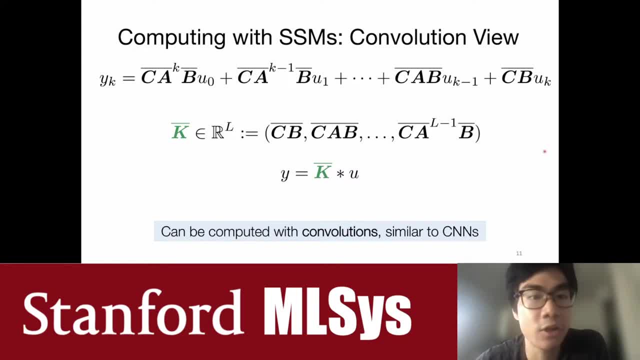 parameters a, b, c, d And by the way, the d term was omitted here because it's not a, because it's kind of like a skip connection that is very easy to compute. And so in the diagram again on the right side here- this is the convolutional view is depicted. 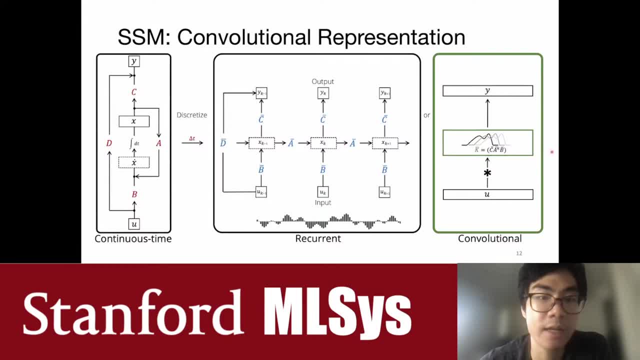 as just you take your parameters and you materialize this convolution filter and then the entire output as a vector can be computed in a vectorized way with a single convolution. Okay, so these are the main properties, So we're going to talk a little bit more about the features of the state space model and how it. 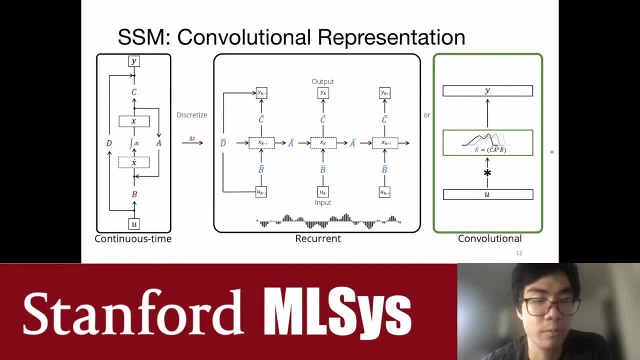 relates to the three types of deep sequence models we saw before: the continuous time, recurrent and convolutional models. It turns out that this is so. this gives a lot of really nice properties, which we'll see later, But there's some critical challenges that make it this. 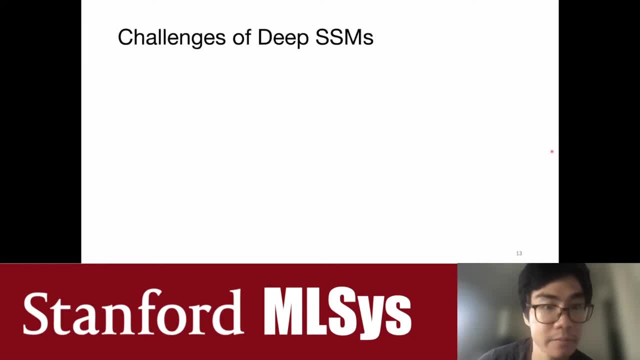 unusable out of the box, And so that'll be the subject of the next few slides. The first challenge is that I mentioned in the beginning that these model families all have problems with long range dependencies, And that's a problem we haven't addressed yet. 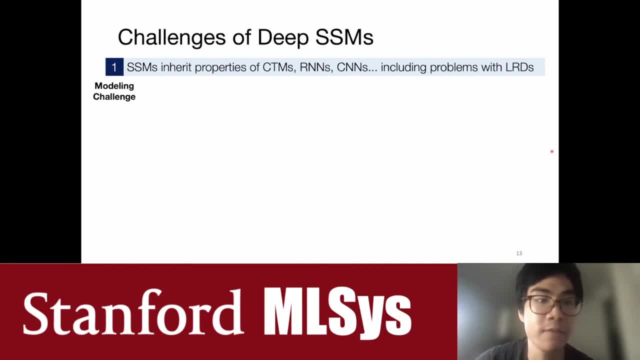 So it turns out that state space models, sort of being a special case of these things, also have problems with long range dependencies. Very concretely, if we look at the state space equation- and in deep learning we usually take these the parameters and randomly initialize them- 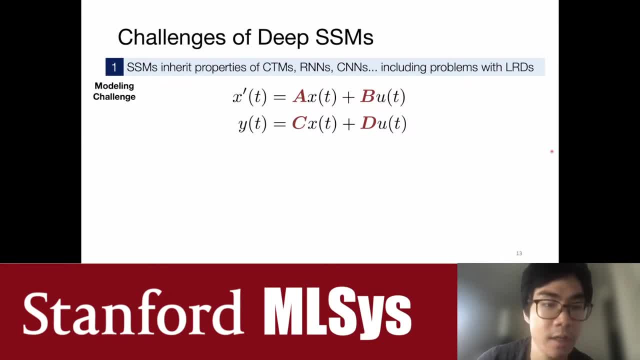 and then start learning them. we learn these A, B, C and D parameters, But if you randomly initialize them, this A matrix is the most important thing in the model And so this is a most important parameter because it controls the, basically the state dynamics, But with a. 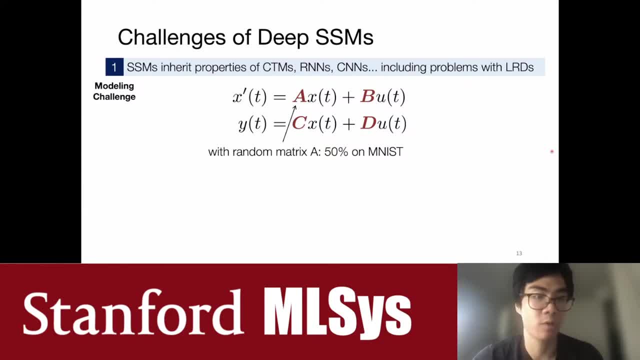 randomly initialized A matrix, this model basically doesn't work well at all. So on the simplest sequential MNIST benchmark, which we'll see later, which most sequence models are expected to do quite well on, at least usually they look at, you expect at least 90% This model. 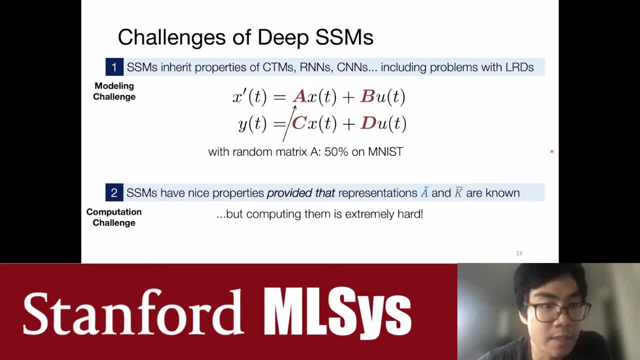 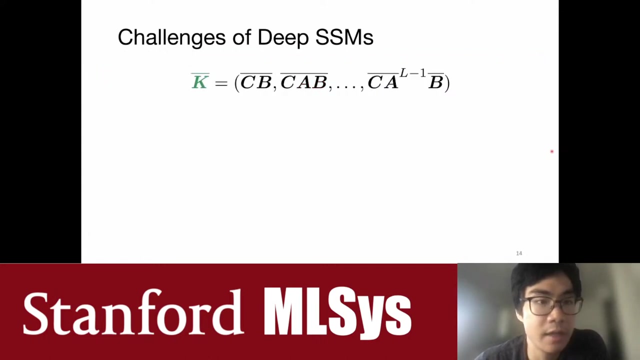 does really poorly. The second problem is that I mentioned that there's three representations of the state space model, and having the representations gives you nice properties, but actually computing the representations, although it's feasible, it's very slow, and so this ends up being a significant bottleneck that makes it difficult to train these models in a little more detail. if we just look at 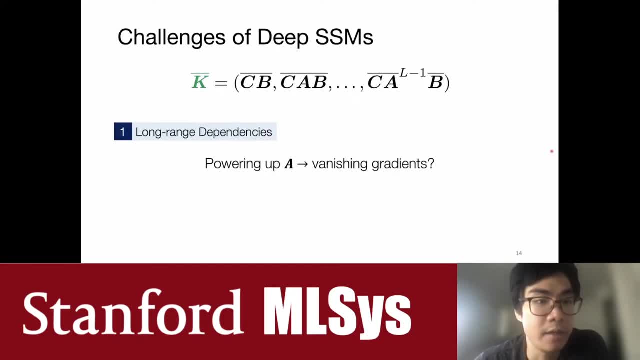 this convolution filter k bar. you can see how the two problems arise, because this convolution filter involves powering up this a matrix, and when you power up the a matrix it runs into the same advantage and gradients problem that i alluded to earlier. and secondly, by powering up this a 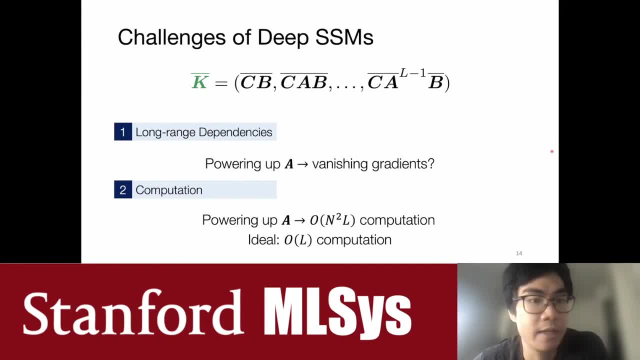 matrix repeatedly. you're doing a lot of extra work to maintain this, this state, and here the sequence length is denoted by l, the state space, the state size is denoted by n and there is a, the odd way of computing. this has a large factor of n extra um we think of our state size in general. 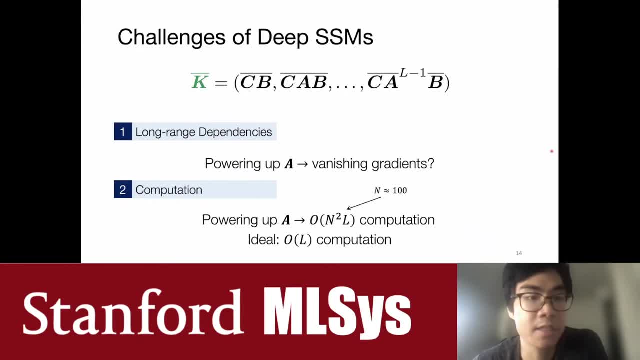 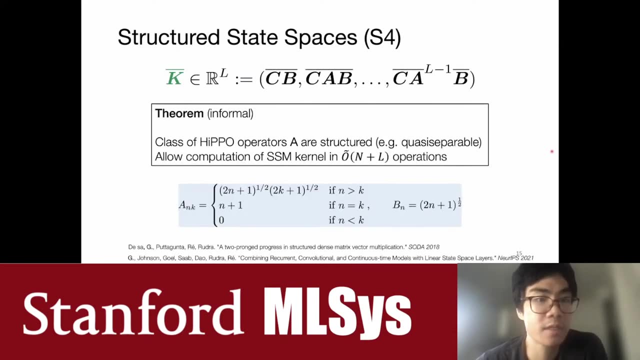 will be on the order of 100 or so, and so this is significantly slower than what you want. it makes it basically unable to train if you use the naive way to compute this. so to get around this, the structured state space model, um, uses some specific uh, add some extra structure um, so there's a. basically we what we do. 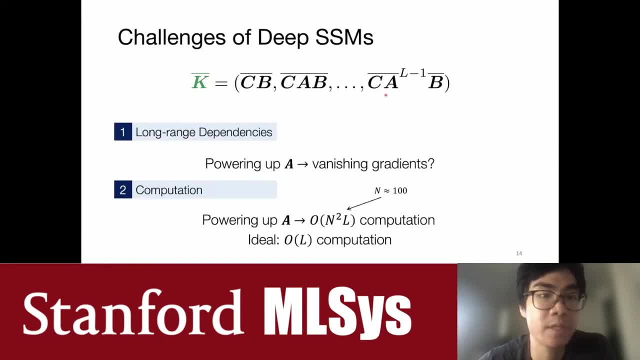 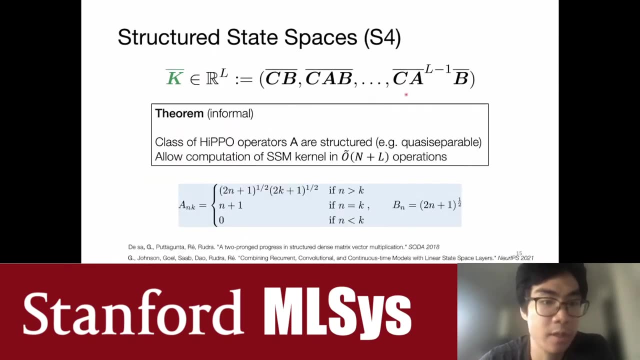 is what we do, is we require a specific formula. we require a specific formula for the a matrix, which is called the um, it's- uh, it was introduced by some previous work of ours, called the hippo theory of memorization, and this specific formula looks like this: um, this formula. 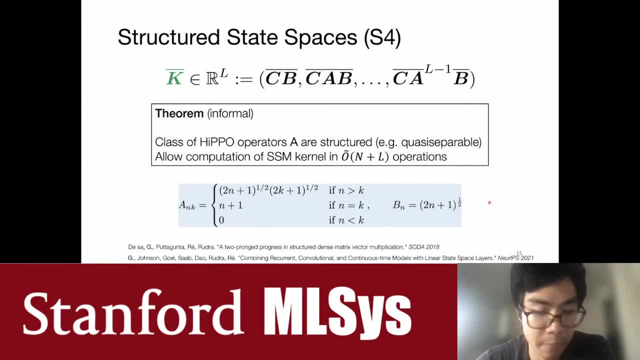 down here and um the this formula was arisen by deriving, by solving some, uh, some mathematical problems involving how to memorize a sequence, and what happens is that if you plug in this precise formula for a and b, then mathematically your state space is trunch- will then be trying to memorize. 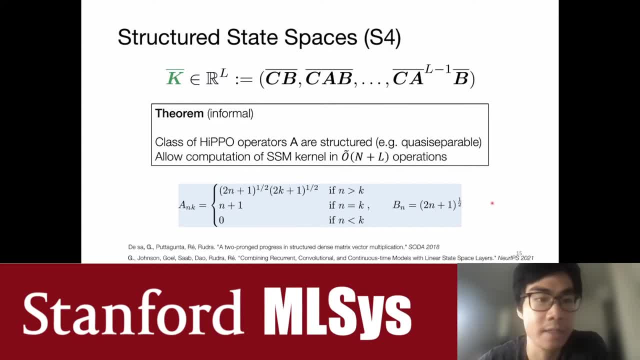 your input signal, which should give it the ability to address long dependencies, um. and so the first thing is that, by incorporating this formula um, our model is automatically able to address long dependencies and secondly, because these matrices are highly structured, it also allows us to address the computational challenges because, intuitively, the idea is that we just need to. 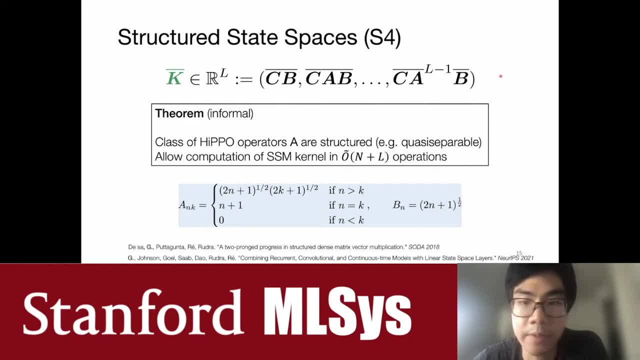 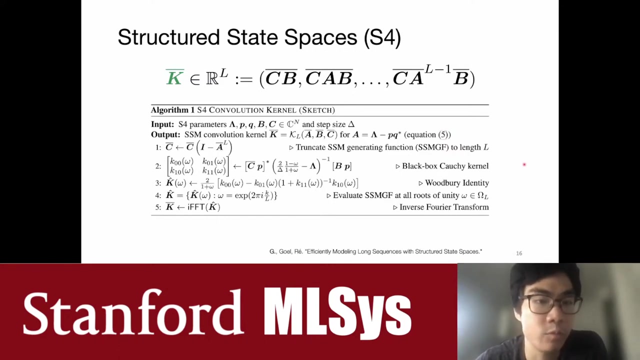 figure out how to compute this thing for this specific formula for a and b, um. and then this formula has a very precise form: um it's. it falls under certain classes of structured matrices and we introduced some particular algorithms that allow this to be computed fast. here's a very high level sketch of the most recent algorithm we introduced. 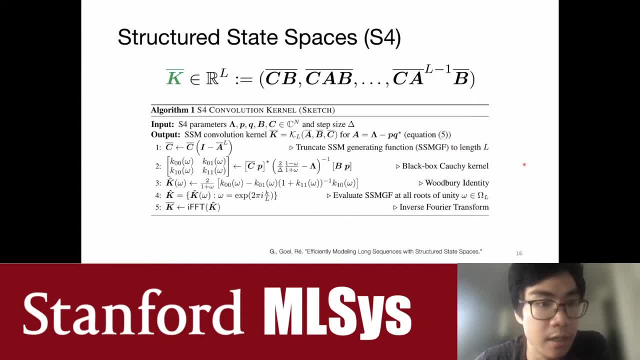 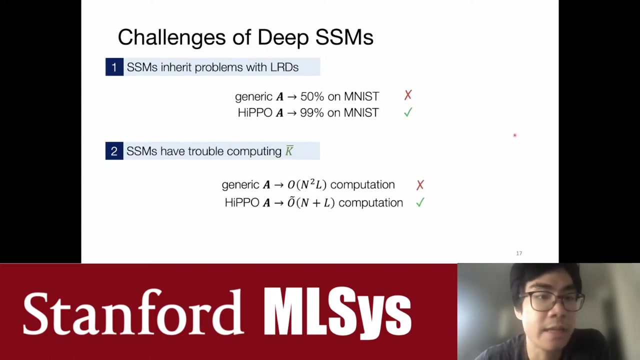 which is the one we use for the structured state space model, um, and basically this allows you to reduce um several fact, polynomial factors in the runtime and this makes it about as efficient as any other, as efficient as possible for a generic sequence model. so, going back to the challenges, um, basically by using that special formula for a introduced before, 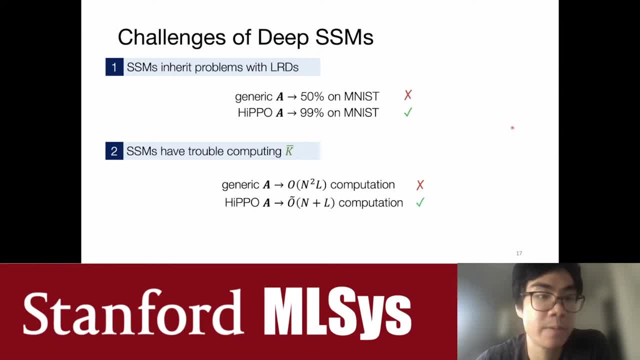 this um the incorporating it into the state space model automatically solves both of the challenges. it um basically goes from very bad performance to basically state of the art on a lot of data sets and it reduces the computation time to make it about as efficient as the fastest competitive sequence models. 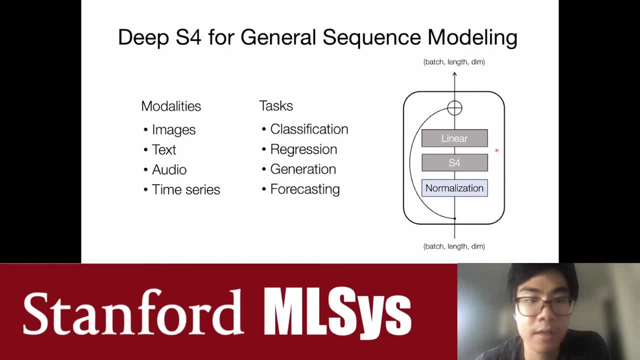 so in overall the um s4 model consists of just that state space model with the initialized to the hippo matrix, using a particular parameterization, and then in our experiments all we do is we just stack them using a very simple repeated block in the same style as: 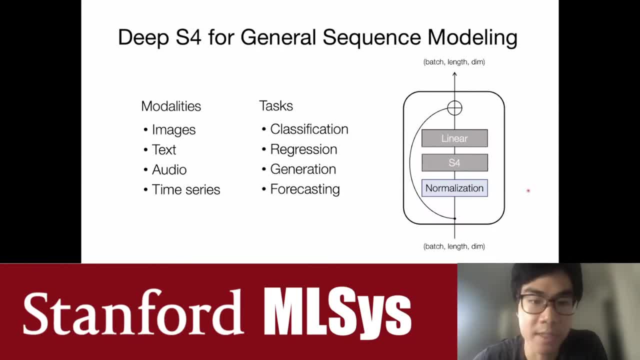 standard deep sequence models. so there's a normalization layer, like later normal batch norm- um, we use that- then the s4 layer, which was, you know, the what i've been talking about, and then some position-wise linearities and non-linearities as well, um, and then, and we've evaluated this model- 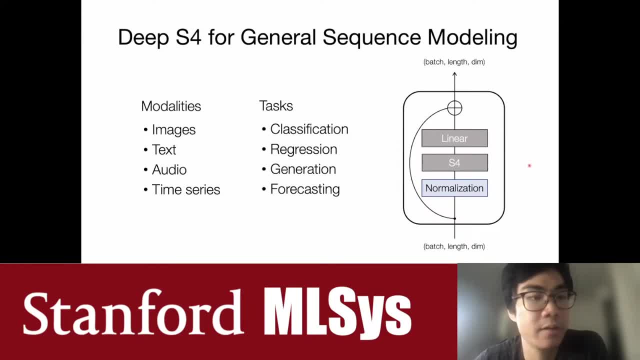 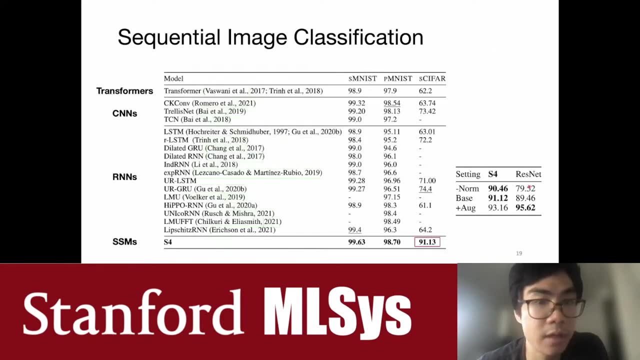 on a bunch of dom tasks across different data modalities and different tasks. um yeah, so these include images, text, audio and time series, and i'll go through a couple of the most important experiments that we've done on the s4 model. so first of all, on uh, we started with one of the most standard 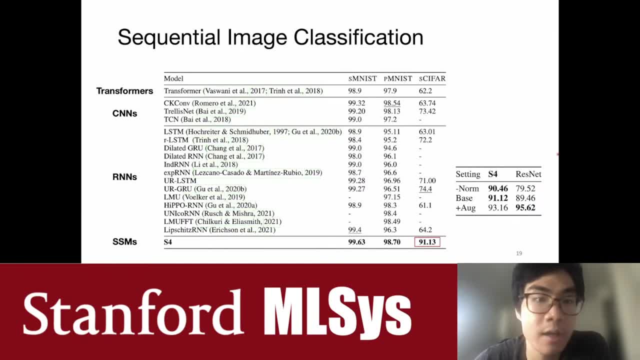 sequence modeling, benchmarks, which is simply doing image classification, but when your image is flattened into a sequence of pixels. so this is something that's been catching on recently in models such as the vision transformer and others, um, but the kind of the most pure version of this is trying to actually, uh, do classification on images purely from pixels. but we're looking at 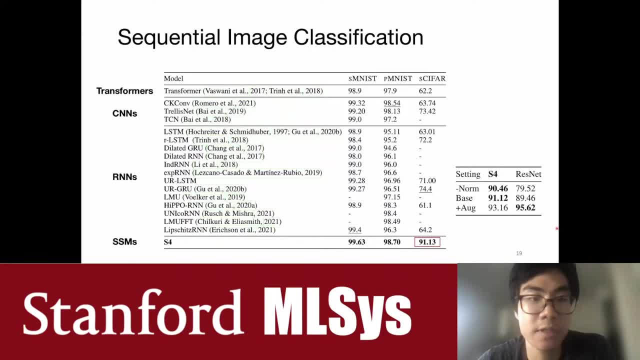 an image sequence that's just a generic sequence of pixels and where the model doesn't know about the 2d structure. now there's a lot of prior work here on a bunch of data sets. the most interesting result here is our result on the sequential cifar benchmark, so the cifar 10 classification. 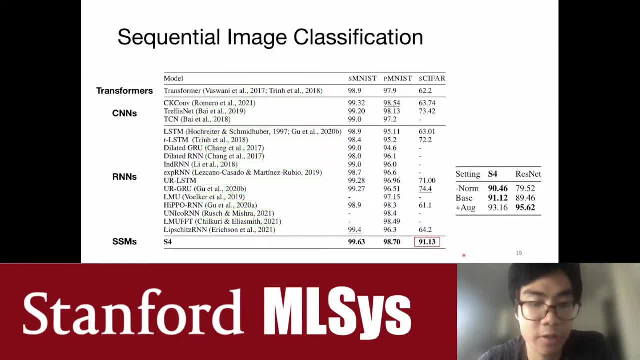 is a 32x32 image and the sequential version turns it into sequences of length 1024, and the s4 model performs 15 to 20, 30% better than all previous sequence models that were evaluated on this benchmark. So it gets over 90%, which in the setting, without data augmentation or anything. 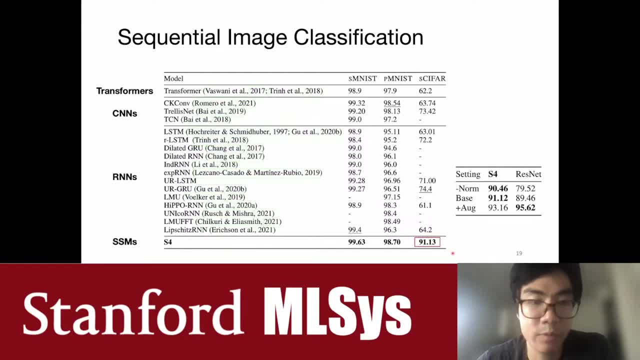 else is actually even better than a simple ResNet-18.. And we performed some other ablations comparing it directly to a ResNet, which is a 2D model, and found that S4, which doesn't even know about the 2D structure of the data, performs almost as well as the ResNet across a bunch of 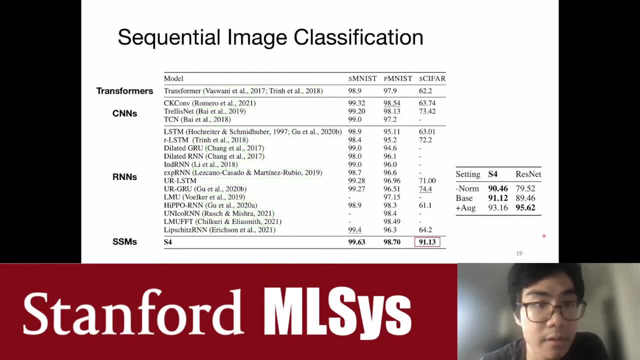 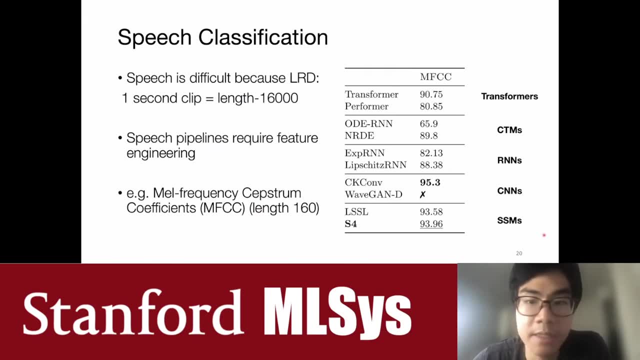 regimes For some more realistic sequence or time series data sets. we tested on a speech classification task, which involves it's called keyword spotting on a data set called speech commands, which consists of one second audio clips that need to be classified into words. 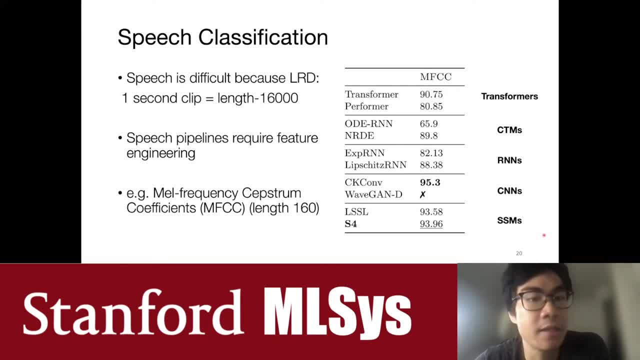 Now, speech is difficult because of the high sampling rate, which makes sequences incredibly long. So here, because we have one second clips, the sequences have length 16,000, which is far longer than most sequence models are designed to address, And so usually speech pipelines require. 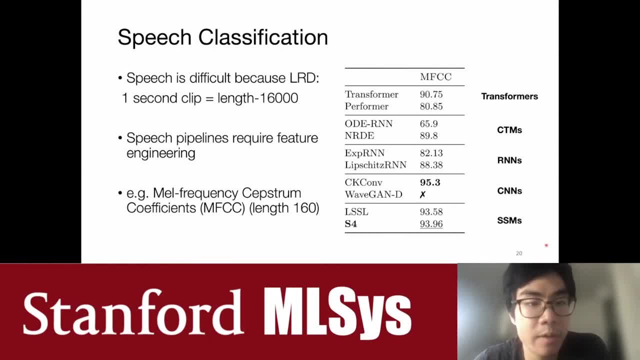 substantial feature engineering. The most common way of doing this is using MFCC coefficients And on this data set, the prior work that we compared against, basically create these filter banks, which reduces the sequence length by a factor of 100, from 16,000 to 160.. And using these pre-processed features, most baselines 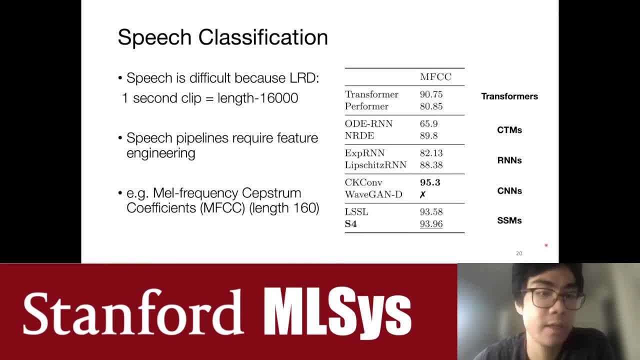 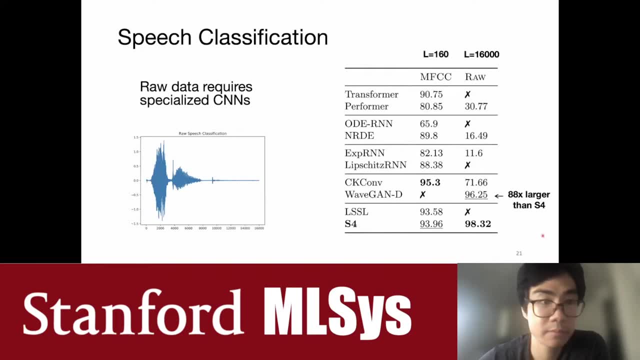 pretty much all sequence models can do pretty reasonably at least 80 or 90 plus percent. The interesting question is how they do on the raw data. So on the raw data, which had sequences of length 16,000,, pretty much all standard sequence models don't work well at all. 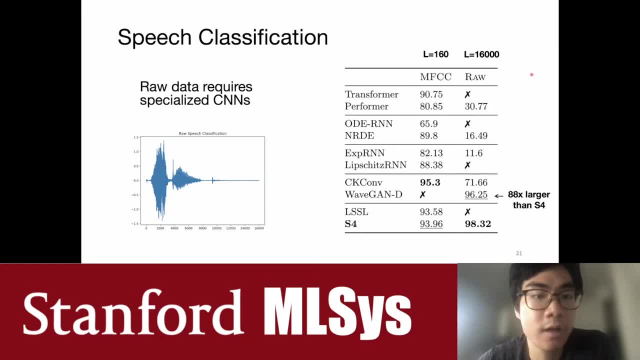 The only types of models that we're aware of that work are the specialized speech CNNs, And we have one baseline here which was designed for sequences of exactly this length for speech. These models can do quite well, but our same generic S4 model. 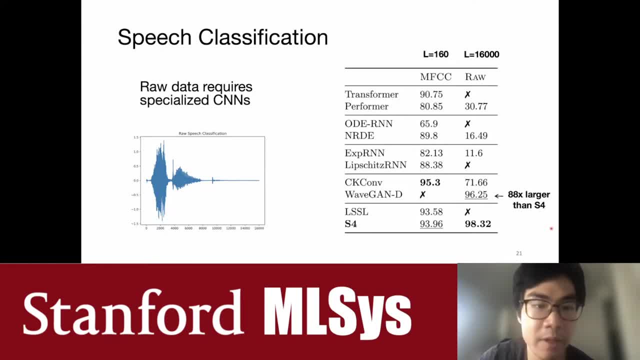 that actually is almost a hundred times smaller than the speech baseline compared against, does even better, And what's interesting is that these models do even better than all of the MFCC models. So this gives us some hope and some future directions for whether we can learn better. 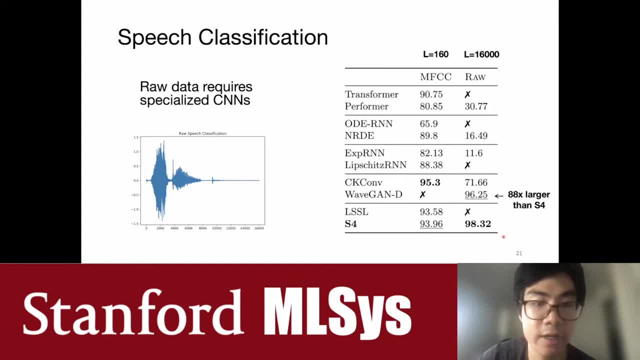 features than the standard speech pre-processing just by using generic deep learning models. The final setting that we tested on this data set is showing that our model can also handle irregular continuous data. So one problem that with working with time series in general is potentially missing value or having a deal with signals sampled at different frequencies. 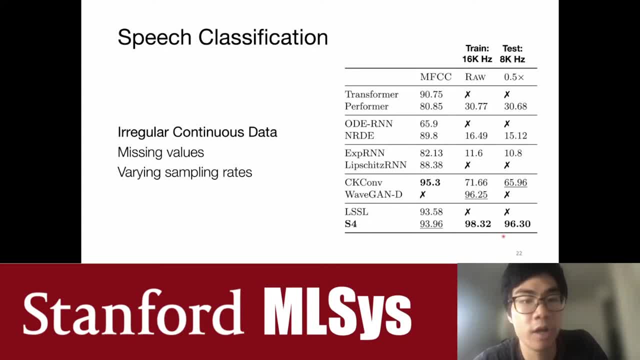 So the way we test this is that we took our same model train on the raw data, which was sequences of length 16,000, sampled at 16 K Hertz, And then we tested it on, without retraining at all or knowing about differently sampled data. We tested it on data that was sampled at 8 K Hertz. 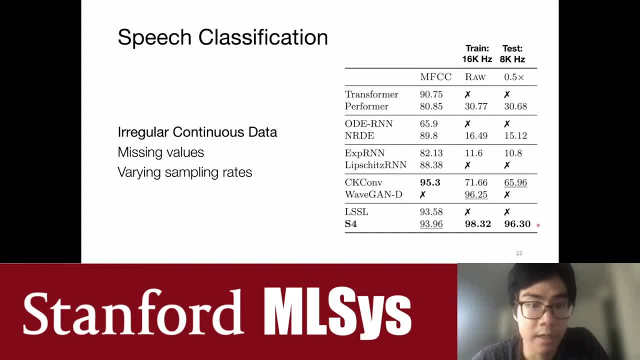 So basically half the sequence length And the other baseline. we compared against the speech. CNN. it doesn't work in a setting but because of properties of the S4 model it actually works out of the box with no retraining on handling data sample at different rates. The reason is because of the first representation. 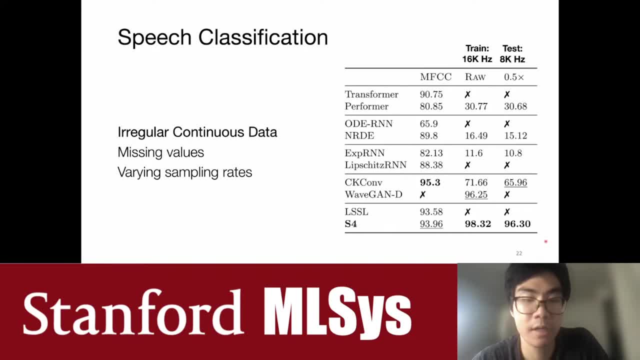 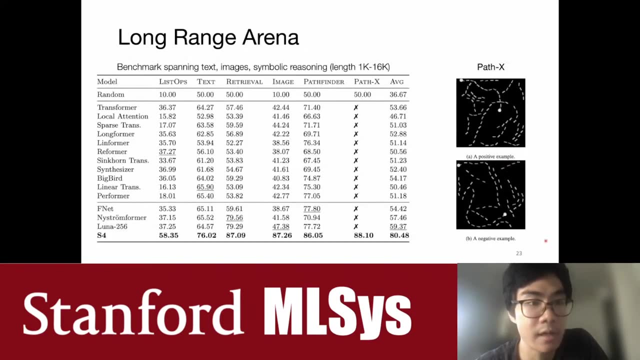 where S4 is implicitly a continuous time model. So it's implicitly modeling not just the sample sequence that you get but the entire underlying continuous speech signal, And this allows it to handle the same signals when sampled at different rates. Here's the long range arena dataset again. 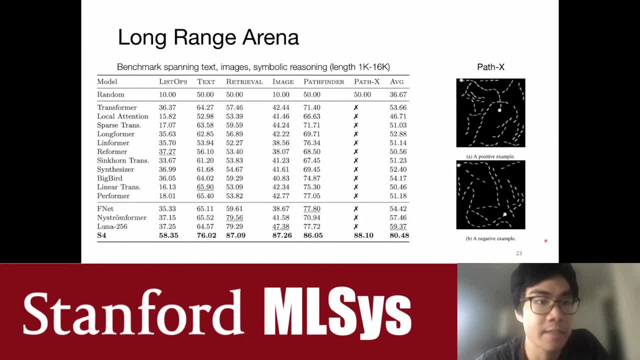 So, again, this was. there are six tasks here spanning all sorts of sequence lengths, And so as a generic, as a model that generically is good at long range dependencies because of the previously mentioned HIPPO theory, S4- again just a simple S4 model. 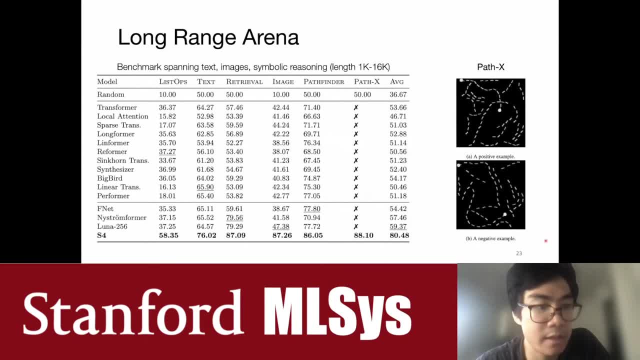 that consists of layers of the S4 block as state of the art on every single task in this dataset. The most interesting result here is the path X task, which is again another image classification task, where you take, you take images- and the binary classification task. 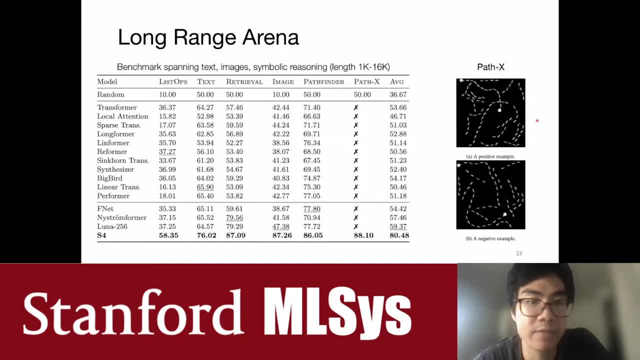 where you have to identify whether the markers are connected. But instead of seeing the image, you just see a sequence of pixels, And because the image is high resolution, the sequence is 16,000 pixels long, And this task is so hard that no previous sequence model has solved it. 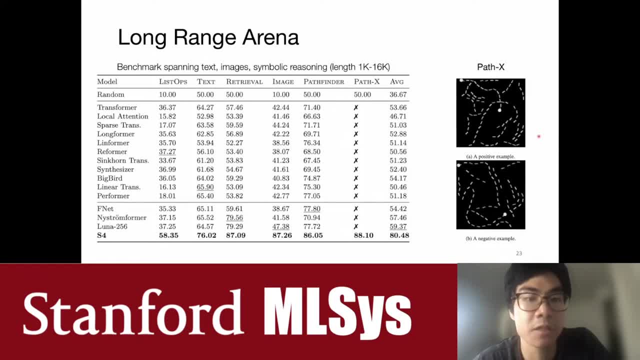 And furthermore, many 2D CNNs also can't solve it. So even like a ResNet-18 can't solve this task if it's given the 2D version. So this is the, I think, our most interesting result: that S4 actually is able to solve the actual. 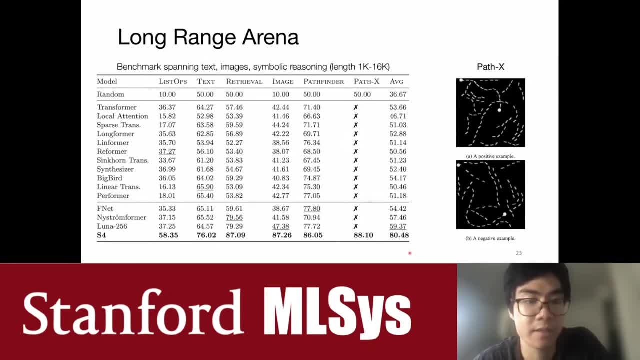 as a generic sequence model, was able to handle the dependencies of length 16,000 here and is the first model to solve this task. This benchmark was also originally used to benchmark the speed of models And, as I mentioned, S4, and there's a typo here. 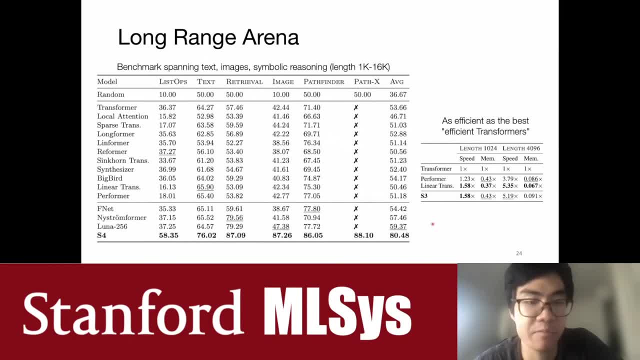 this: the model was renamed from S3 to S4 at some point, if people are confused, But, as I mentioned, we have particular representation algorithms. that makes S4 very efficient And it's as efficient as every other efficient transformer model that was comparing this benchmark. 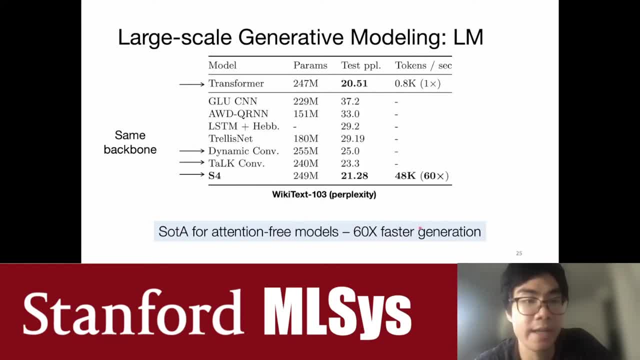 And finally, we showed that S4 works, has promise, on text as well. So text is an area where transformers are dominant instead of RNNs and CNNs, And by taking a transformer backbone and swapping out the attention layer for S4, we show that it's quite close to the baseline. 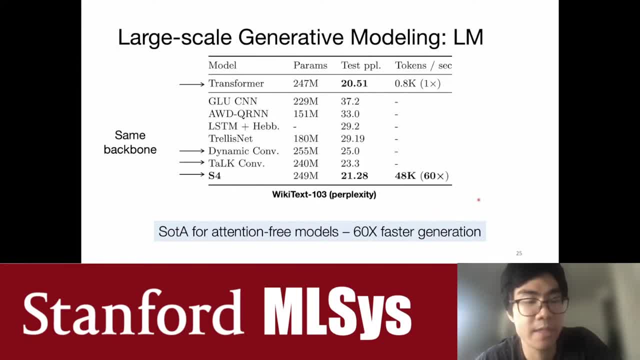 less than 0.8 perplexity off, And this is actually a substantial state of the art for attention-free models. Furthermore, by leveraging the RNN representation of the model, the trained S4 model can generate do auto-aggressive generation much faster. 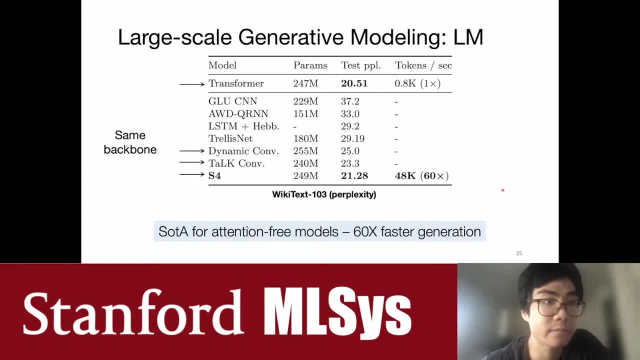 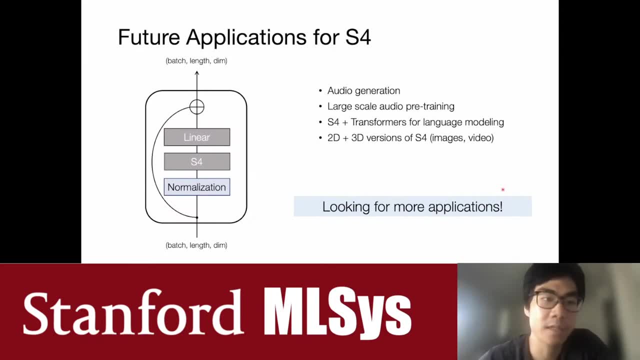 than alternative models like the transformer. We are investigating many, many more applications, including something I alluded to earlier is: how can you learn better features by perhaps doing large scale audio pre-training? We are looking at more generation tasks, So, instead of language, can you generate audio by itself? 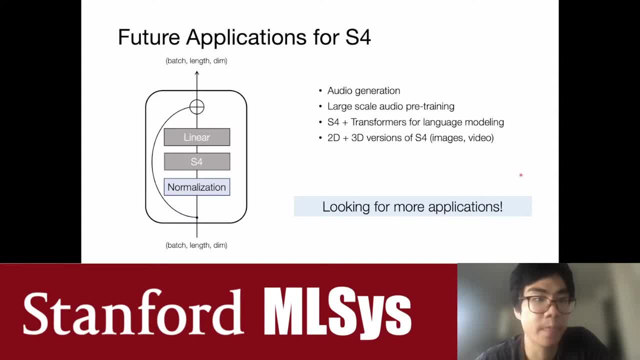 and leverage the faster generation properties. We're interested in combining S4 with other models to do better on language and other domains, And we're still thinking about theoretical extensions of the theory to 2D or higher, And this may allow it to address modalities. 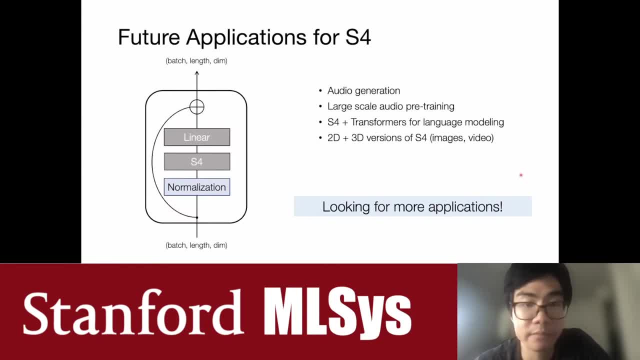 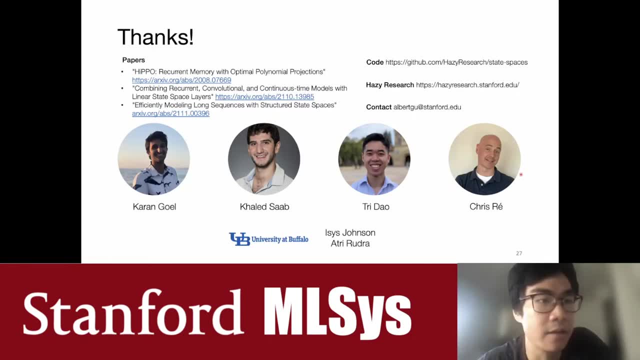 such as images and video, more naturally. That's all So we have. this work was based on three papers that I mentioned: the HIPPO paper, which introduced the mathematical framework for memorization, which was the basis of the long range dependencies. 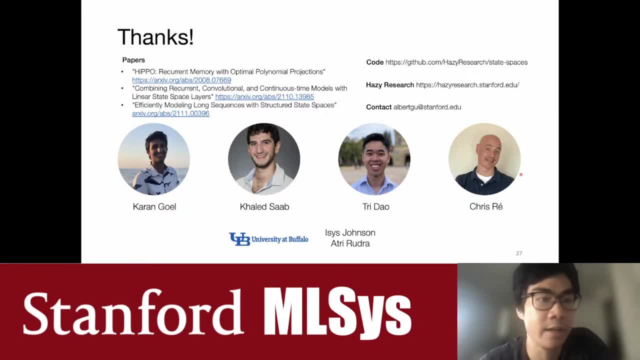 and then two works on state spaces that culminated in the S4 model. Our code is online And yeah, and thanks to all my collaborators, Curran, Kale, Tri and Chris, my advisor, from our lab, Hazy Research- 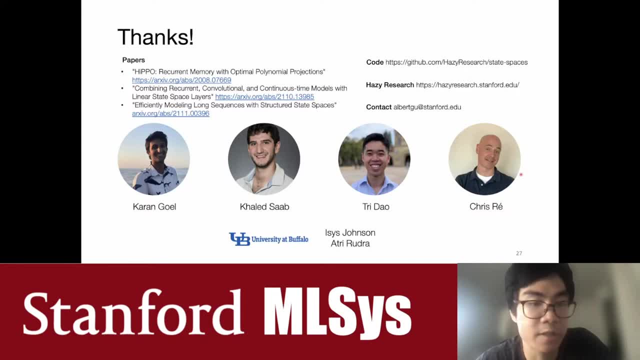 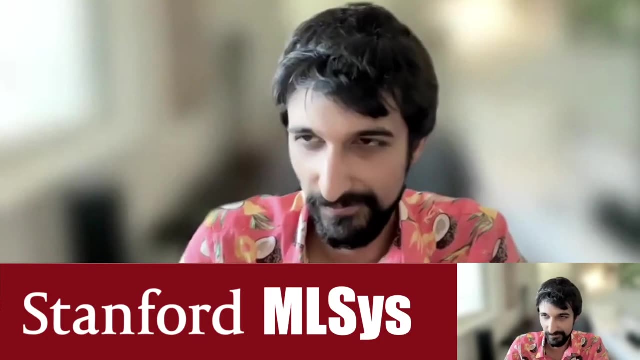 as well as external collaborators Isis and Autry from the University of Buffalo. Awesome Thanks for the talk, Albert, And we have a bunch of questions in chat And a quick reminder to folks in the YouTube chat to keep posting questions. Yeah, so I guess to kick things off. 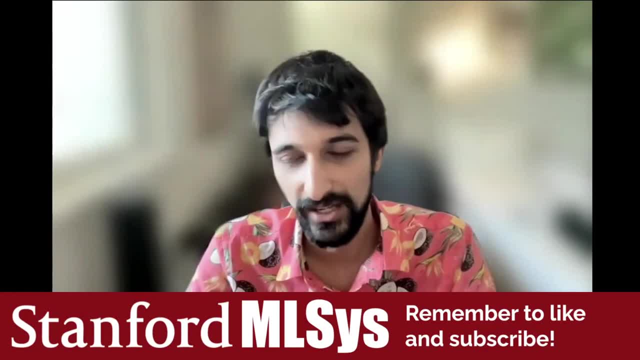 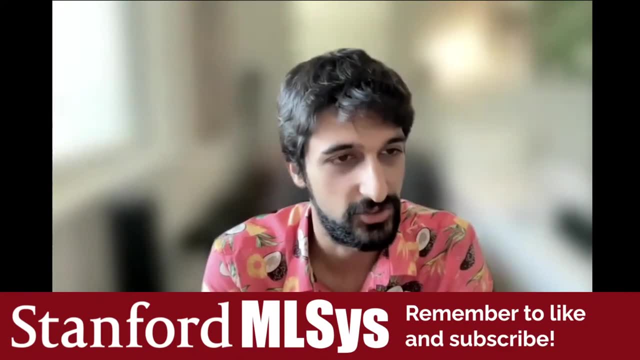 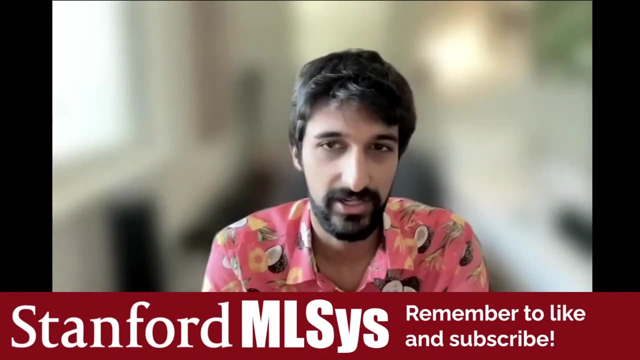 I'll just grab a question from chat, because we got quite a few. One set of questions, I think that were asked from Chuck was about the A matrices and whether the A matrices are constrained to be stable and whether sequences generated by all stable A matrices would lead to zero final state. 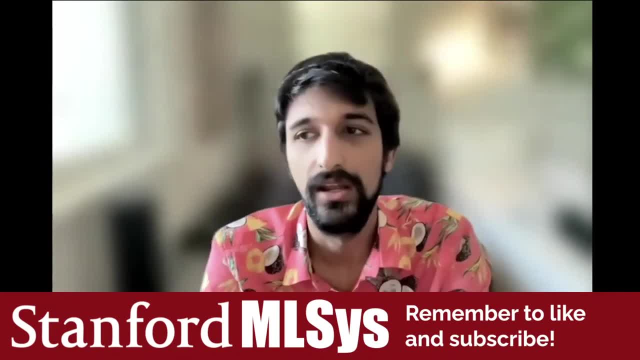 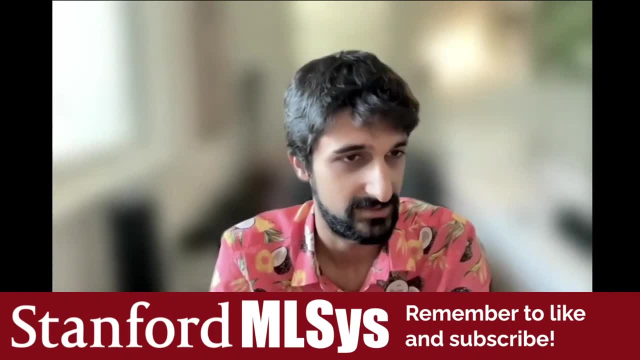 So that was one question And I think in general there was a question about whether these A matrices need to be derived from the hippo theory to memorize the sequence, or if they can just be any stable matrices. Yeah, these are great questions. 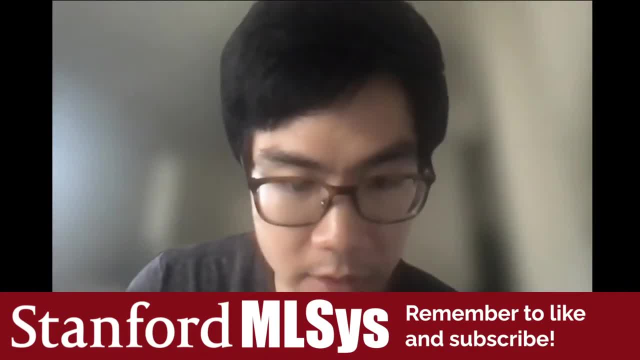 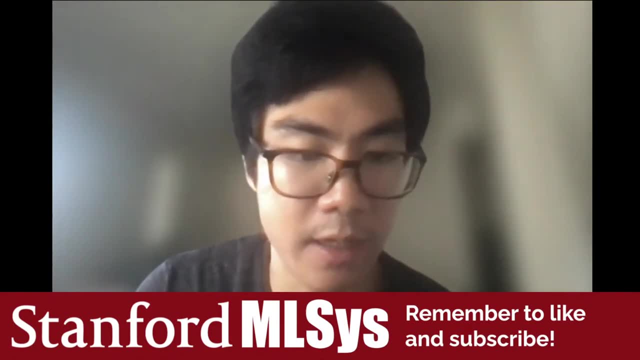 So let's see. So the first question is: do the A matrices need to be stable? No, I'm not sure exactly what stable means in this context, But I would imagine that what you mean is: is it kind of close to unitary? 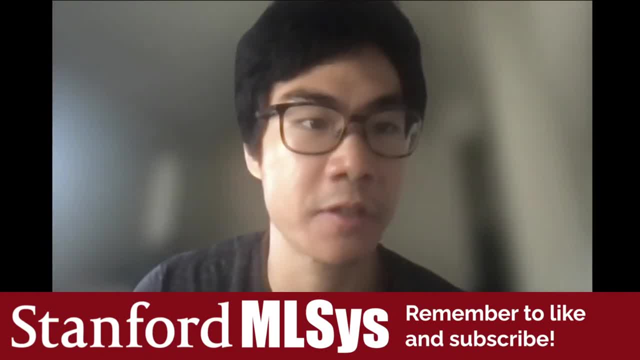 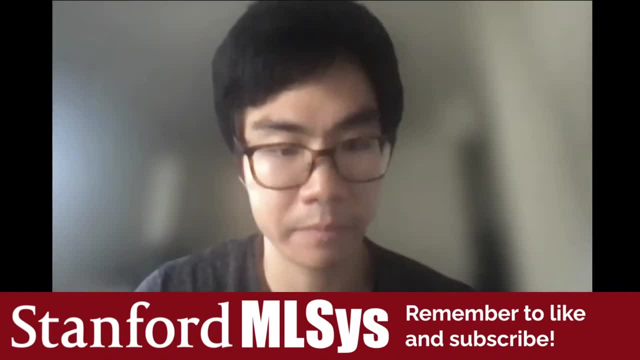 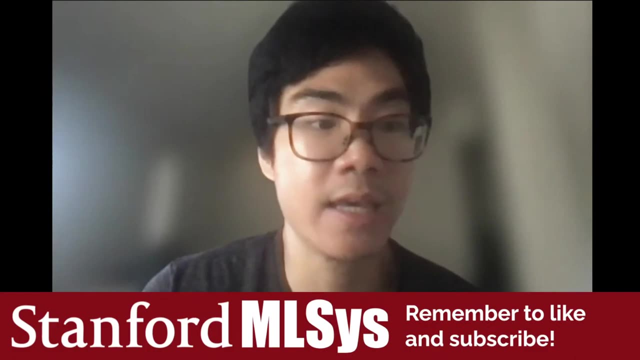 Like? are its eigenvalues and singular values controlled, so that when you power it up it doesn't blow up, which is the main cause of the branching grains problem? So first there's kind of a question and a converse asked here. So first of all, is the hippo matrix stable? 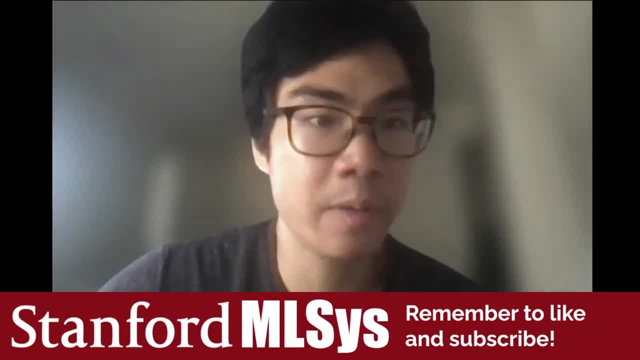 Here's the formula again. The answer is a little bit more. We can't see the slide, Sorry, Just a quick note. Oh, you can't see the slides. Am I? is that on purpose? Yeah, I killed your screen share. 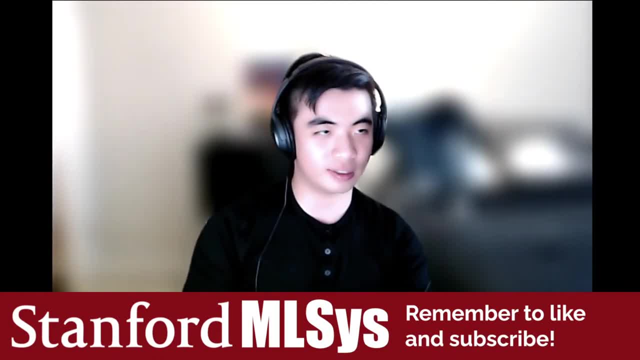 I think we can get it back if you want. But if you can answer without, OK, that's fine. I can answer without. Yeah, the answer is that the stability kind of comes from not necessarily a matrix itself, but from discretized. 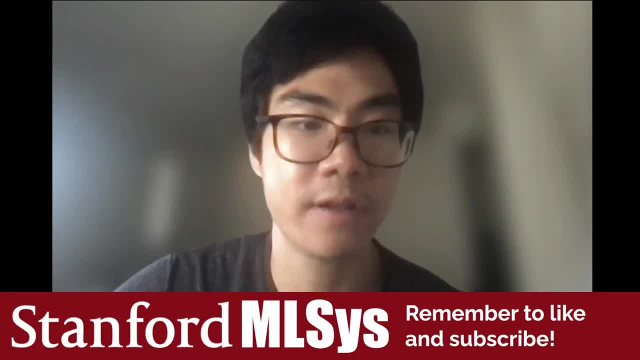 the discretization. So it's kind of both The matrix itself well, kind of by fiat, of the by solving this memorization problem. it has to be stable because it's doing what it was derived to do, which is memorize. 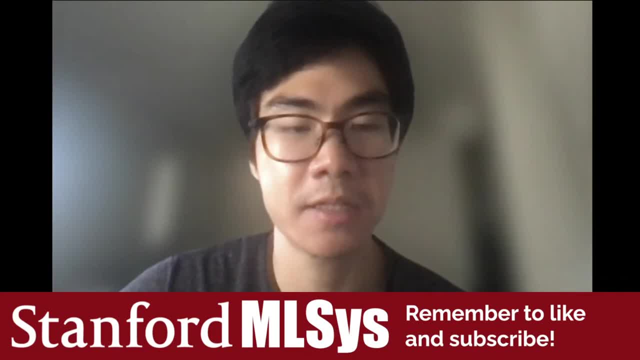 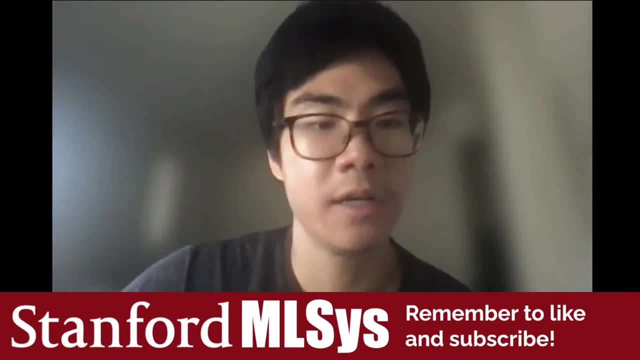 And because you have to be stable in order to address these long dependencies. it is stable. Conversely, though, not every stable matrix will do well. So, in fact, the example result I said where, if you randomly initialize the A matrix, does it work? 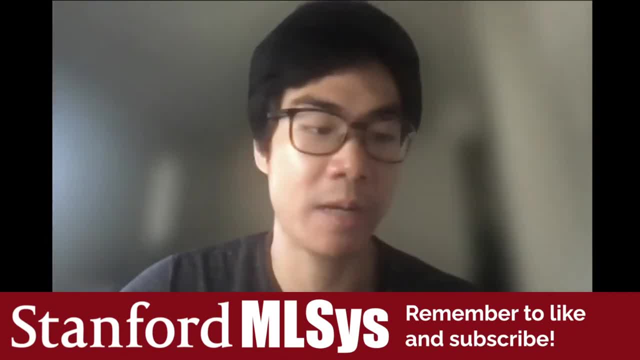 There's actually a little more subtlety there. So, first of all, if you actually randomly initialize it the way you normally do, it will kind of it will NAN out. actually It will give you NANs. It just is completely unstable. 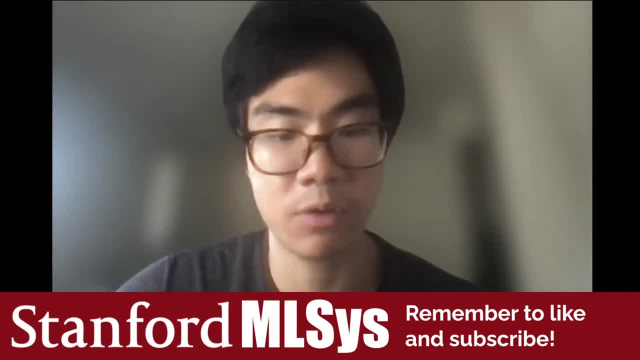 So what I had to do was kind of control the matrix to be more stable by controlling the eigenvalues of it to be closer to 1. And by controlling that sufficiently it then becomes stable enough to actually train. But when you do that then it actually 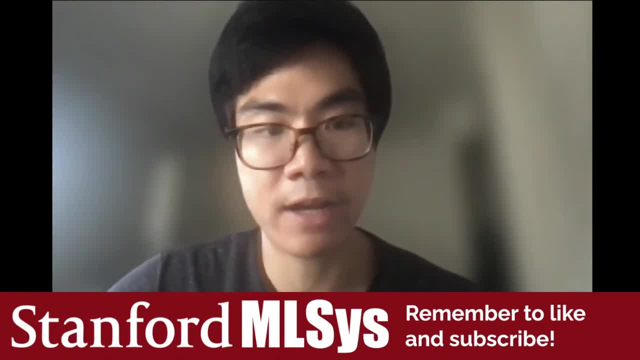 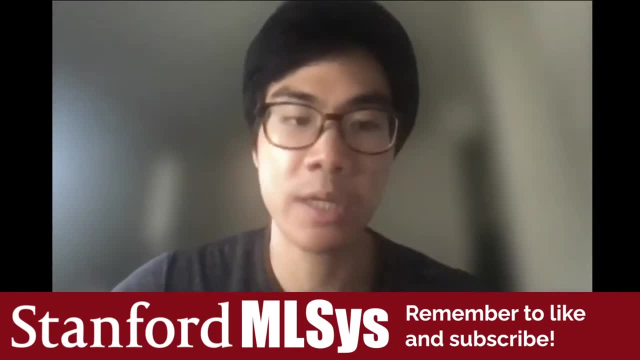 just doesn't perform well. So in general I've actually found that the performance of S4 is really closely tied to the hippo theory. So even if you make small changes to these special formula for that A matrix, it usually substantially affects the performance. 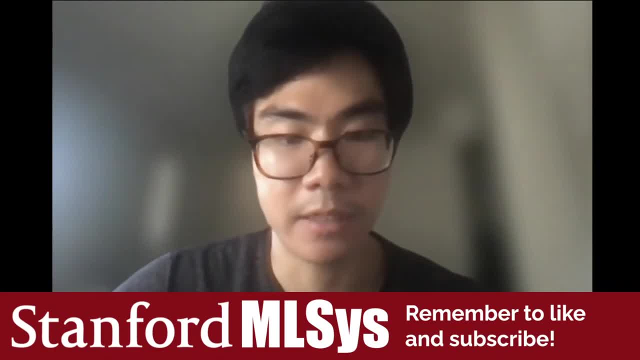 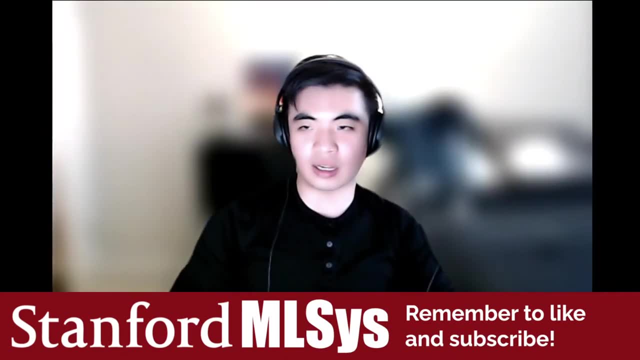 of the downstream model. I hope that answers the question. Yeah, I think. yeah, that's a great answer. So I'll take another question from chat. I think you started to talk about this a little bit at the end, But Adrian in chat is wondering for kind of general NLP tasks. 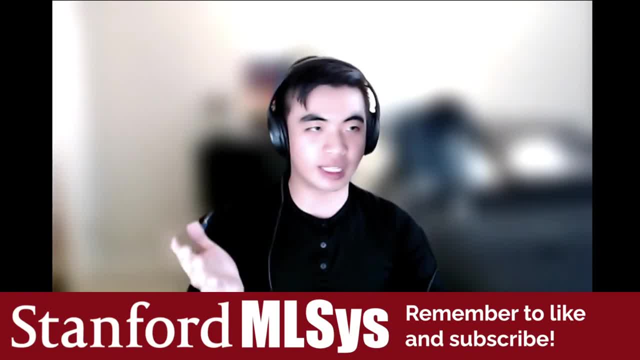 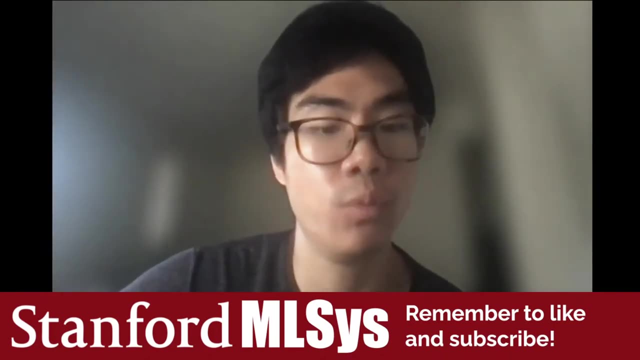 like the glue, benchmark or super glue. have you considered using S4 for these? How would you expect them to do in kind of traditional NLP, kind of classification tasks? So we have actually only considered, I think, S4 for these. We have considered that one test language task, the Wikitex 103. 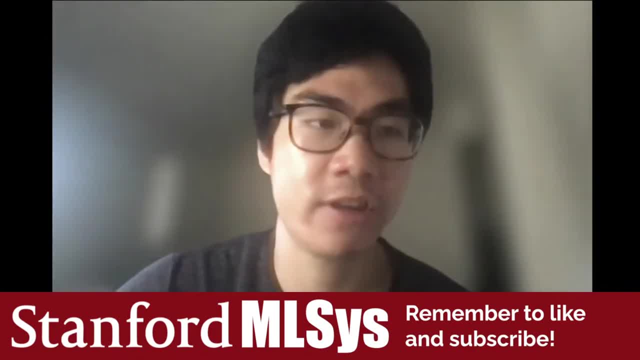 language modeling benchmark And actually, well, I think there was one other classification task inside the long range arena benchmark or the suite. We are quite interested in using S4 on other NLP tasks, including glue, I think was one candidate that we are looking at. 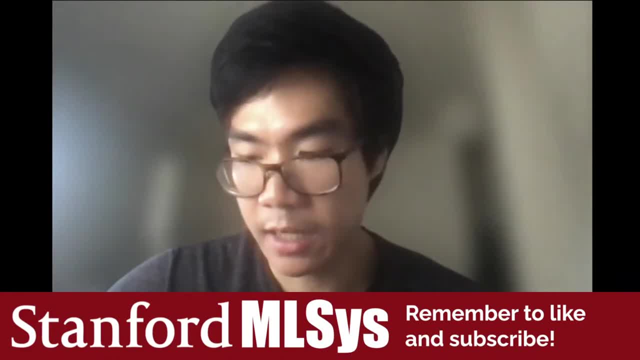 But we don't have any preliminary results. We haven't really tried it yet. This does raise a good question, which is, I guess, something I kind of left out And the talk, which is: what are the limitations of S4?? 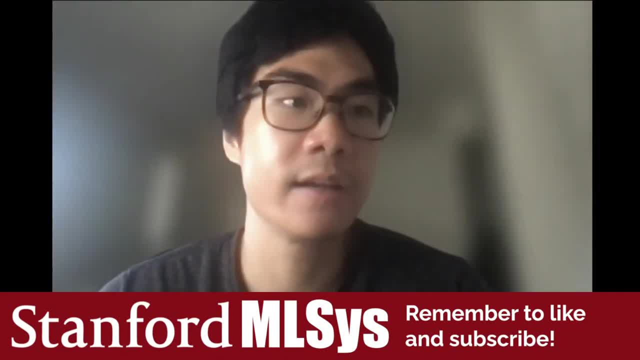 I think that's an interesting question, because we do think that text may be one of the more difficult domains for S4 to address, for the reasons, for an intuition laid out at the beginning of the talk, which is about how it's more designed for continuous data. 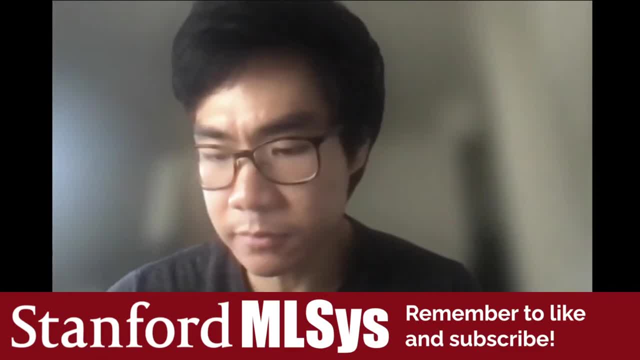 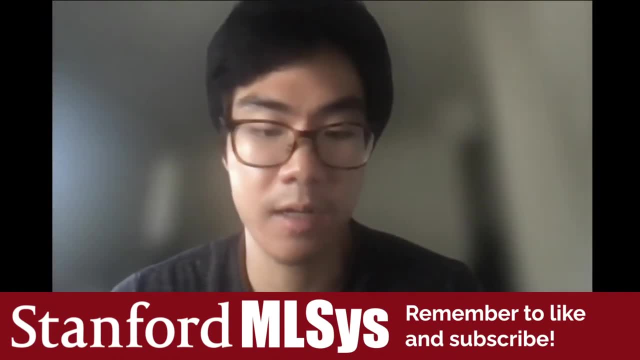 whereas text we view as kind of very discrete data. So we were actually not quite sure how it would do at all. It did better than we expected on the language modeling benchmark And that makes us think there is potential there. But it may be the case that it's more effective when combined. 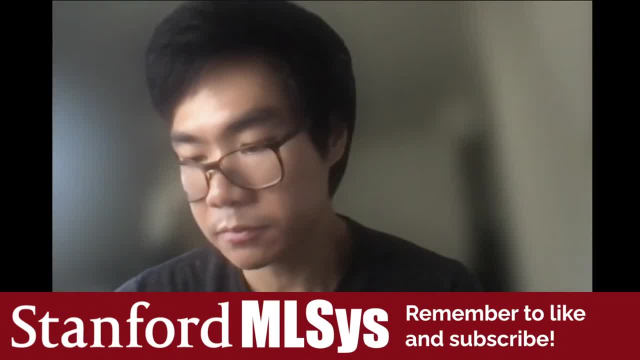 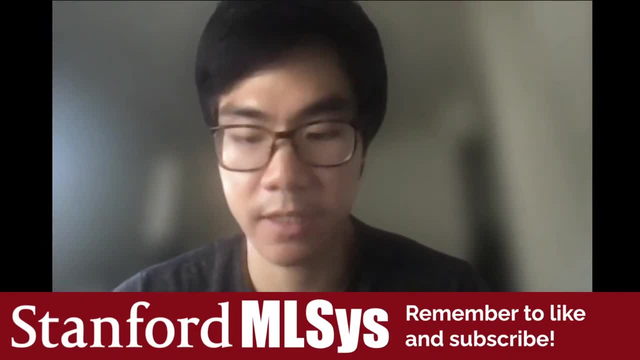 with transformers or other models, Or maybe it just works out of the box by itself. This is something that we actually haven't investigated too far into so far, but it's definitely on our plate. But I actually think that testing on Glue and SuperGlue- 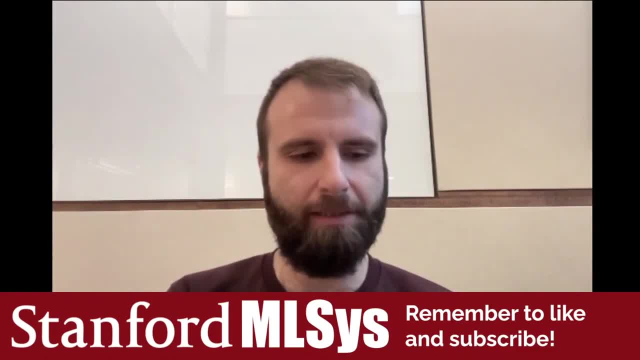 will be interesting to see the properties on those data sets, obviously, But at the same time they don't stack me as data sets where long-range dependencies are particularly like. it's a particularly fitting property of those data sets, right? On the other hand, I think there are other tasks in language. 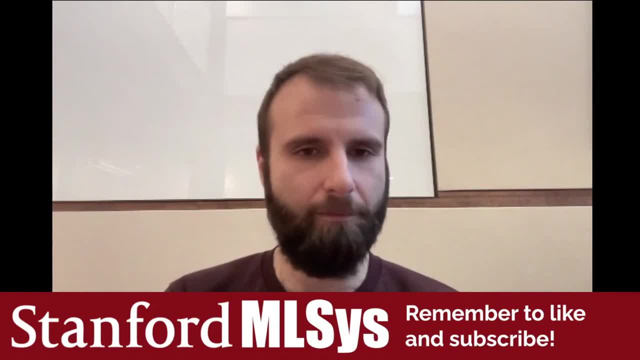 that where I believe it could be really interesting to apply them for this model on, In particular, if you're familiar with the data set as a whole, narrative QA, where you basically have a full book as the input And then you have to do some question answering. 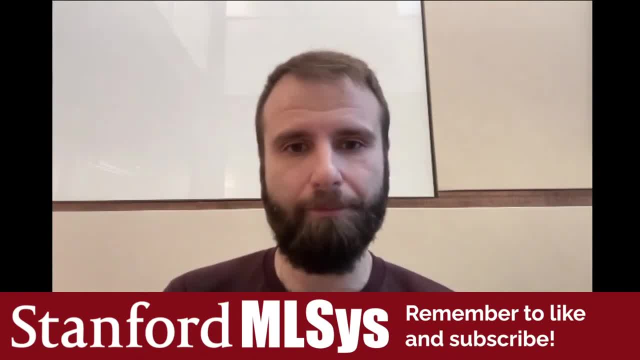 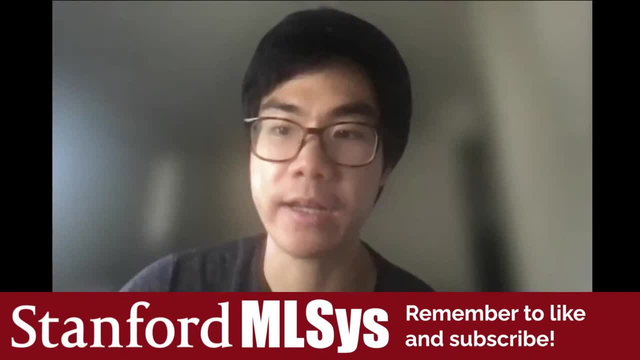 or some prediction. You think that those tasks would be more better, for the model would perform better on those tasks instead. Yeah, great point. I think that's definitely something that we're like. that's the most promising area that we want to look into. 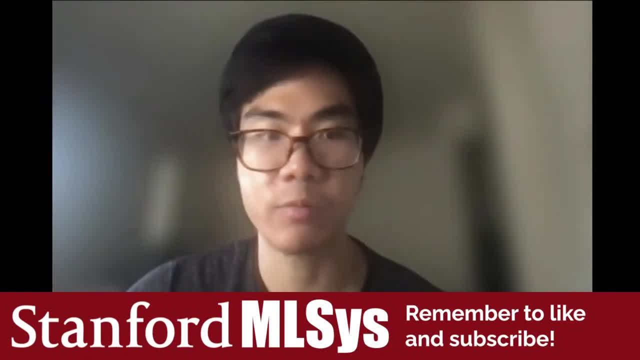 I think there's a bunch of, like I said, summarizing entire documents or books, Or there's other types of tasks such as in context- learning is something I was talking about with somebody just yesterday, actually- where you try to use an entire data set as context. 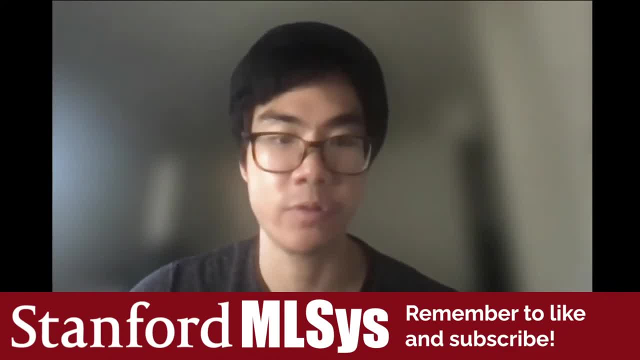 But if you are just encoding it as a generic sequence, then you need a powerful sequence model that can handle these long-range dependencies. There's certainly lots of applications, I think, where this could end up useful in NLP. Yeah, looking forward to your next paper. 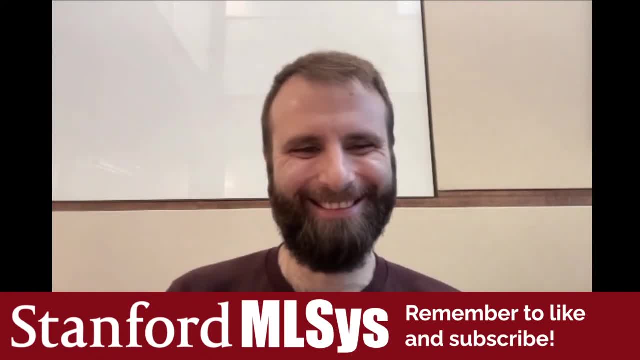 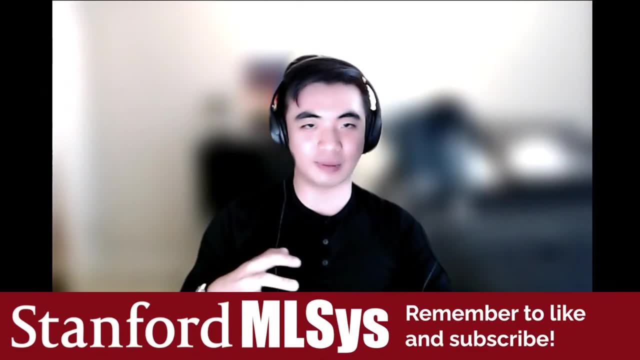 where you tackle these tasks specifically. Albert, one of the things that I personally really like about this work is hearing the story of how you came to develop and dig deep and learn all these things throughout the arc of your PhD. I wonder if you're comfortable sharing with a wide audience. 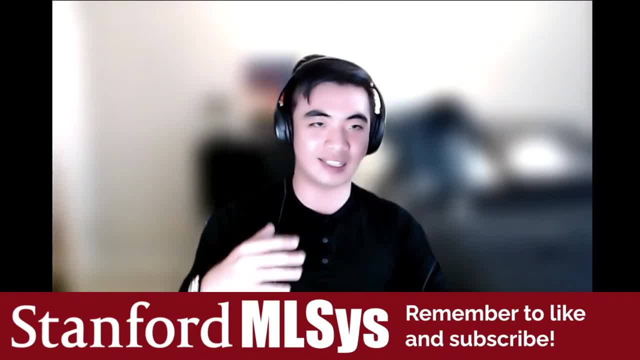 if you could talk a little bit about what that story looks like And, as you are in your last year of your PhD, what advice would you give to younger students- maybe some of us included- who are just in the middle or the beginning of their PhD journeys? 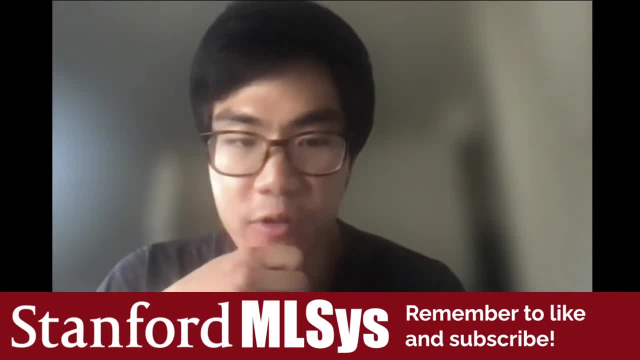 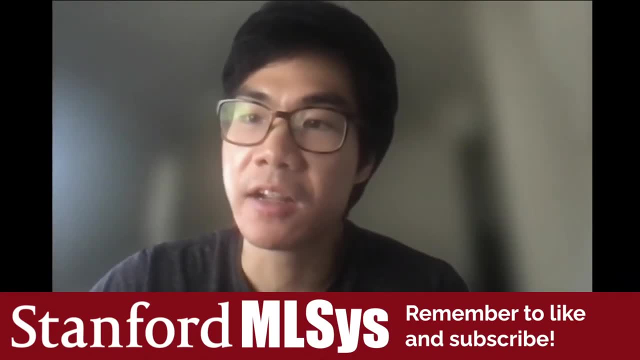 So I can tell you how the pieces of this particular project kind of came together and how that developed. I actually spent a large portion of my PhD working purely on these, This theory of structure matrices. So I mentioned that. the S4 model, one of the key challenges. 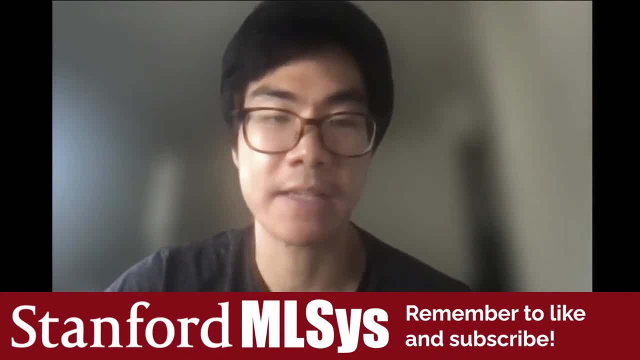 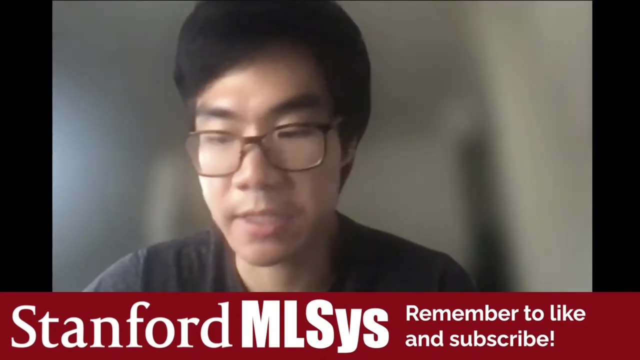 to make it work was developing this special representation and fast algorithm to make it efficient, And that was based off of some expertise I guess I developed in earlier years of my PhD, which was purely on algorithmic aspects of linear algebra structure matrices. 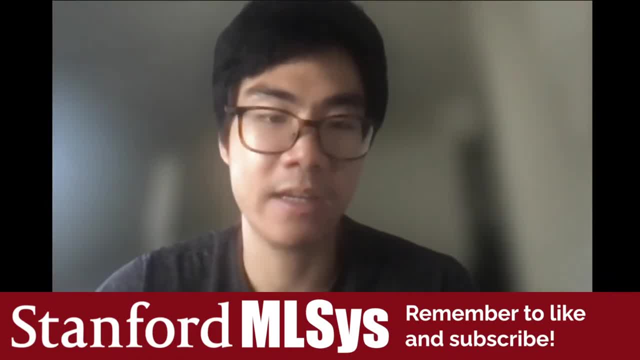 And I had nothing. I never thought that, to be honest, I never thought it would ever be useful, And it was just doing it for its own sake. So the way I talked about this project was that we motivate it from this state-based model, which 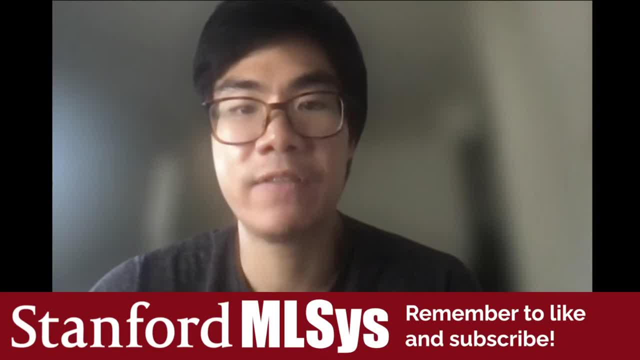 is a well-known model, and then we incorporate the HIPPO theory. Actually it kind of developed in reverse, where we were solving this HIPPO problem of memorization first, which leveraged some of the toolbox we developed on structure matrices, And then we developed the HIPPO model, which leveraged some of the toolbox we developed on structure matrices. 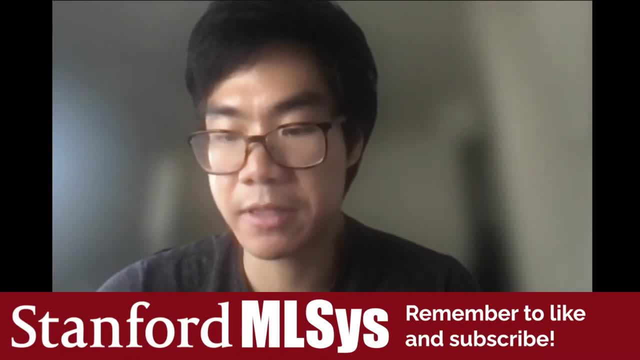 And then we developed the HIPPO model, which leveraged some of the toolbox we developed on structure matrices And we're talking about polynomials and so on, And we came up with a nice theoretical result, but we had trouble making it very effective. 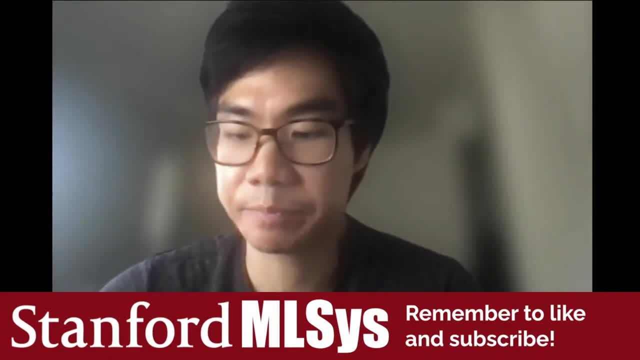 And then the connection to state spaces kind of developed as almost like a pattern match. But it was like we're trying to figure out how to make this work And it turned out there was a natural connection to state spaces that then we investigated and tried to incorporate it. 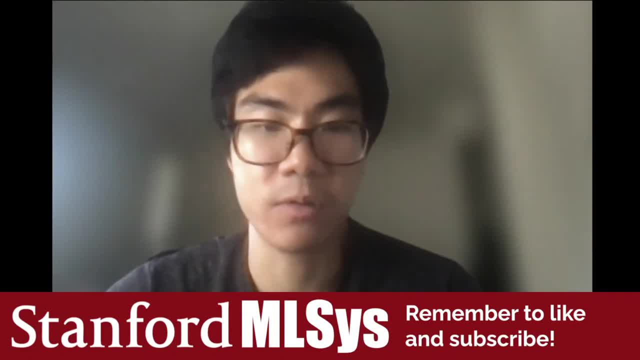 but then ran into these other challenges of the computation and so on. So the final project, I think, is- I mean this work, I think is quite the connection to state spaces is extremely interesting, I think. But it didn't quite evolve quite that straightforward. 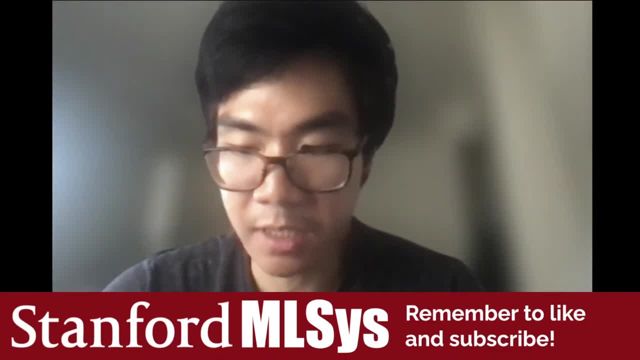 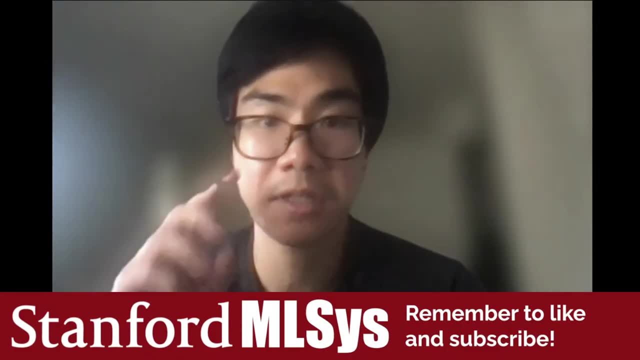 It involved going through these detours, involving lots of just like pure theory and algorithms, and then some math problems on signals, and then finally developed into a method And I think generally that's an experience I've had with research. So to answer your question about the advice, 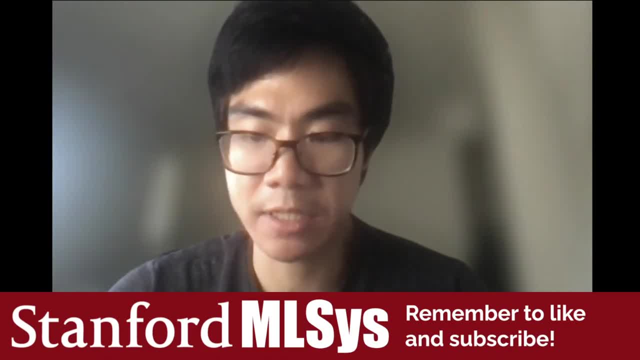 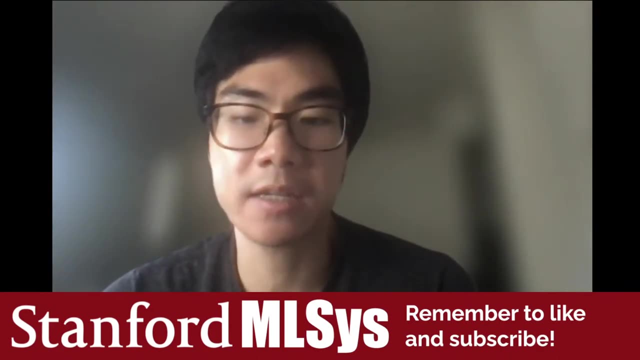 I do think that spending an amount of time on just fundamental tools or investigating just yeah. So for me it was structure matrices, which is kind of like theoretical tools for its own sake, as long as they're interesting- And if they're interesting, then usually you'll find some way. 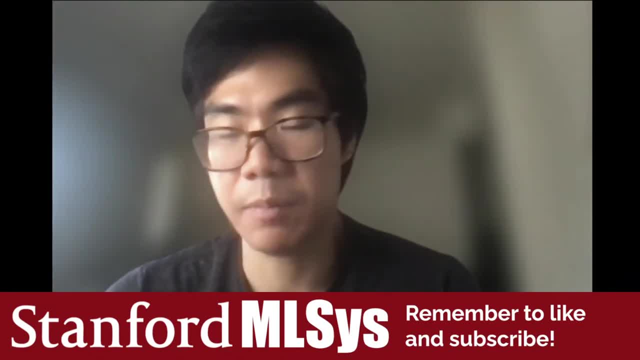 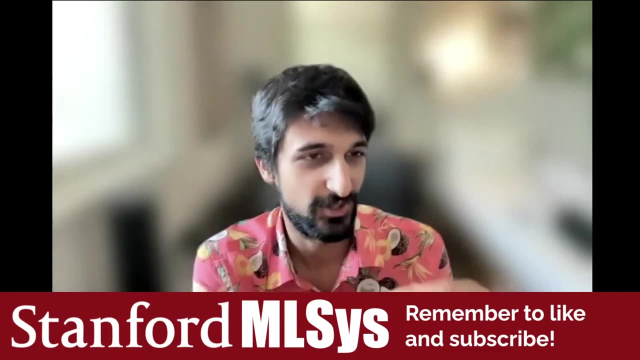 to apply it, And so for me that naturally became applied into HIPPO and then finally into the S4 model. So yeah, that's a great answer. I'm also I'm curious about other, as you were talking through the connection to state spaces. 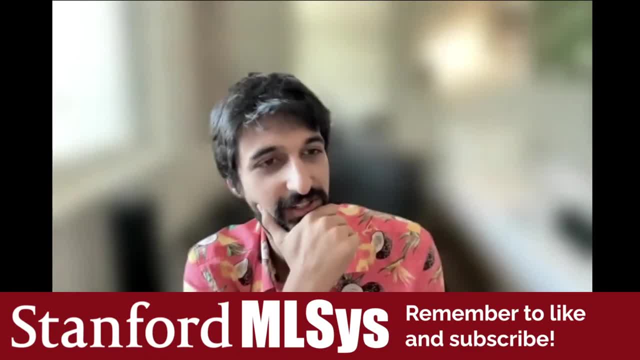 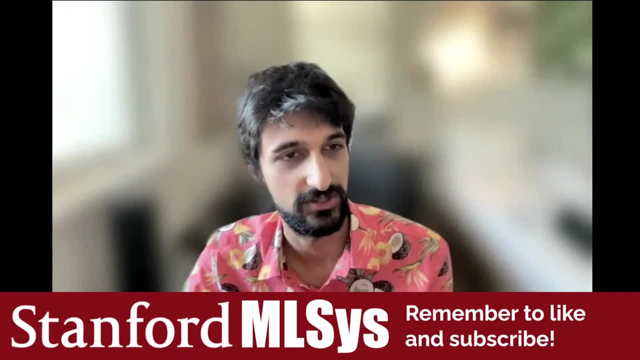 and so on. I'm curious. in particular, I think this also relates to a question we got in chat about other ways to view these state-space models. So, for example, I think one question that Connor had was about looking at other function families. 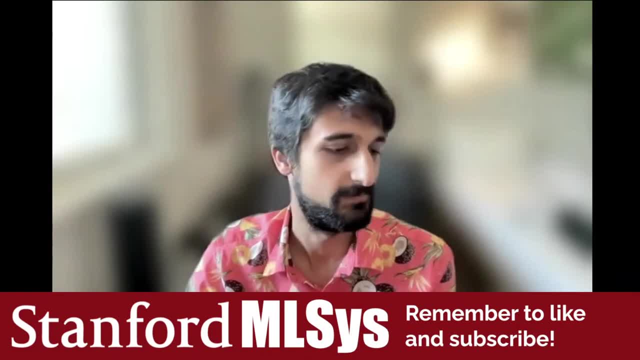 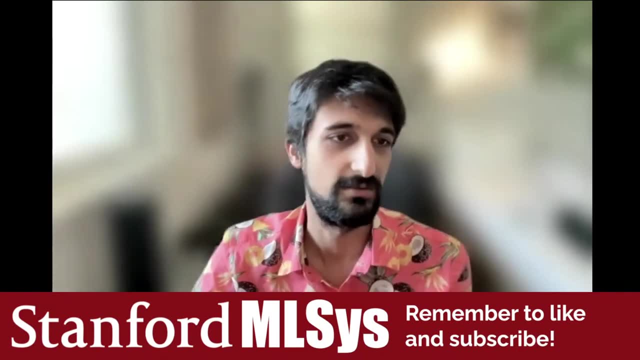 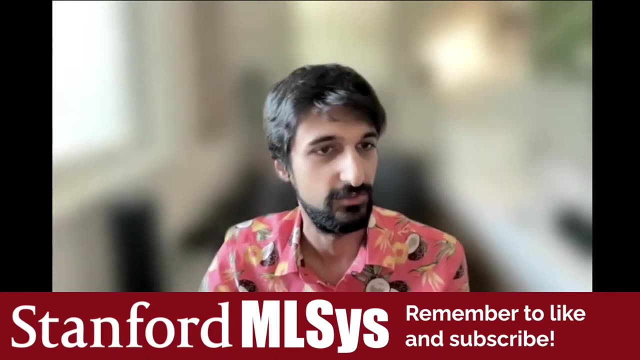 For example, rational functions are in general like the HIPPO memorization theory as well. I know you and I have chatted about this- but other ways to memorize sequences that don't necessarily rely on the particular polynomial families that you consider in this work. 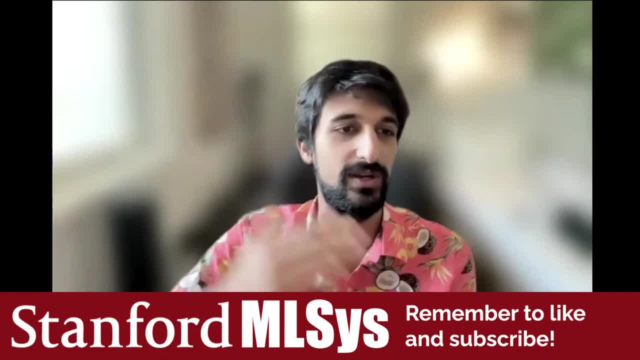 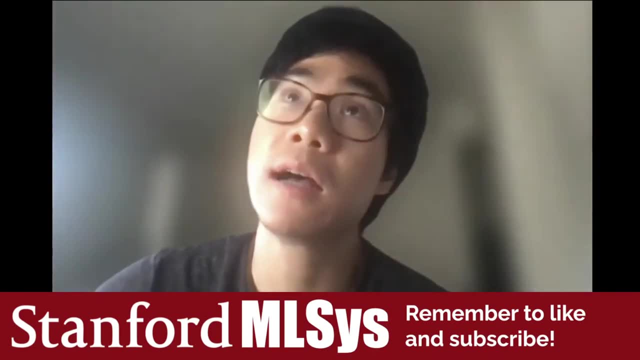 Can you talk a little bit about those? and just generally, how would one extend this into other directions? this work, Yeah, Yeah, Yeah, Yeah, We could work into other directions. So that's a great question. So I think that there's a couple of these. 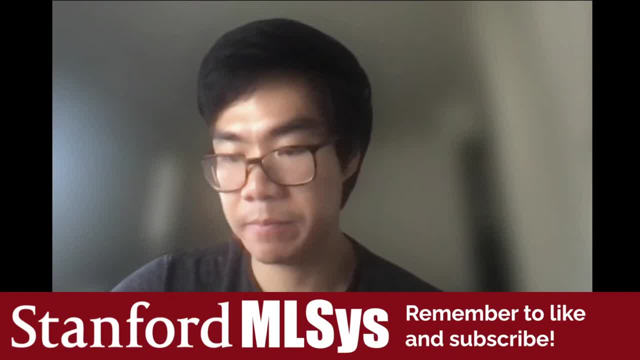 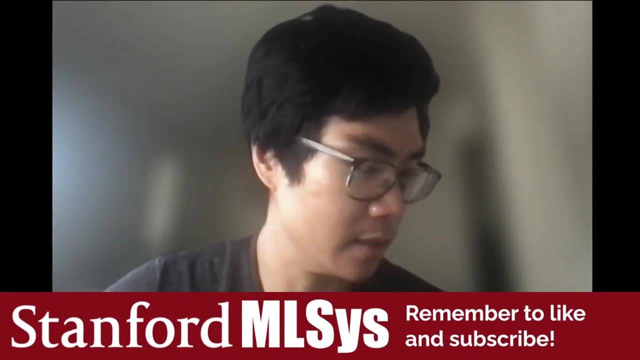 that we're working on ourselves actually And kind of, as Connor identified, I guess one of the cruxes of the glue that makes this work is that theory of memorization, the HIPPO thing, And there's lots of open questions about how to use it. 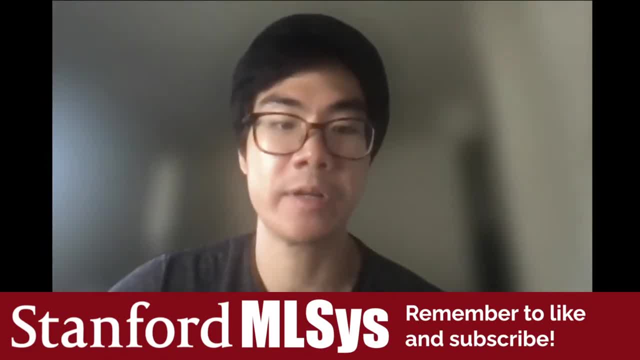 So we formulated a very particular problem that involved approximating functions using like polynomials or these orthogonal polynomial bases, But definitely there's a lot of other bases that can work too. So one generalization that we even thought about was that if you use sine cosine bases instead, you should be able to get some sort of online Fourier transform like method that might give you another, like a different, approximation. 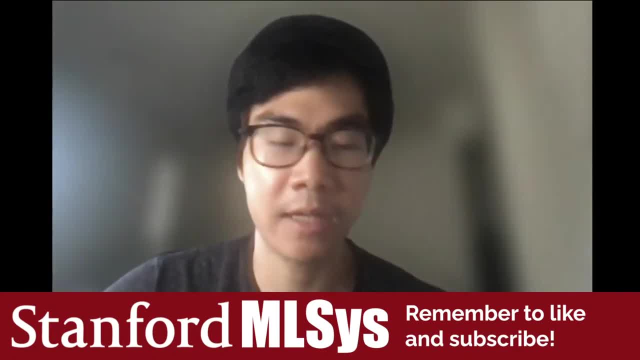 We're also looking into. I guess this is going kind of into the details of HIPPO, which not everyone's familiar with, but there's like it's based on this concept of a measure that can be that's kind of almost a hyperparameter that can be learned over, or there's a there's different. HIPPO wasn't actually so in the talk. I kind of said HIPPO is this one matrix. 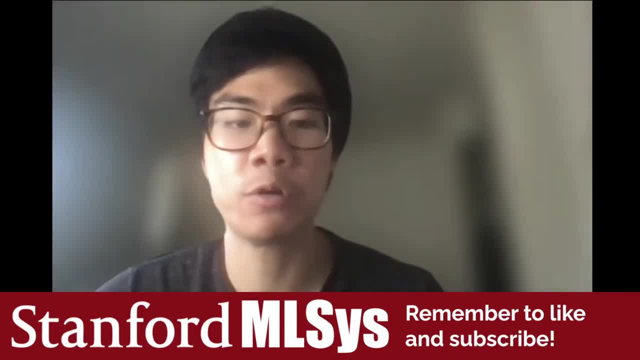 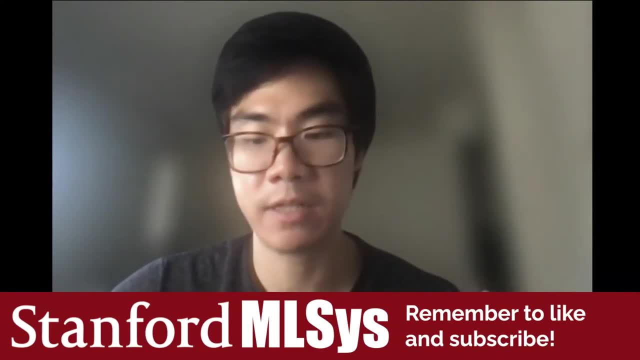 It's actually a family of things, And we don't fully understand it. We don't fully understand every single piece in that family. yet There's ways of using different measures or different approximations that actually might make it better, And that's something that we're currently working on as well. 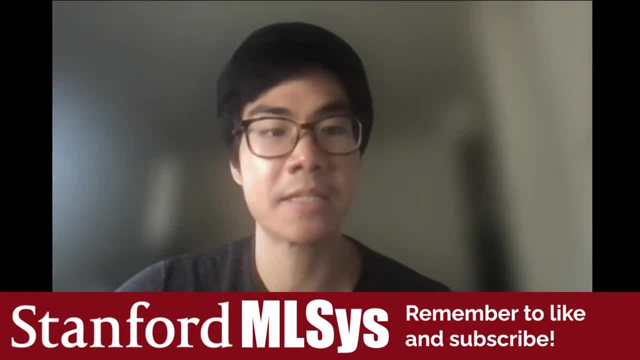 So certainly in terms of like, I don't think necessarily HIPPO is the only way to do it. Like you might find some of these extensions and call it something else, But I think, I do think that having this very clear theory underlying the method, with a formalism of 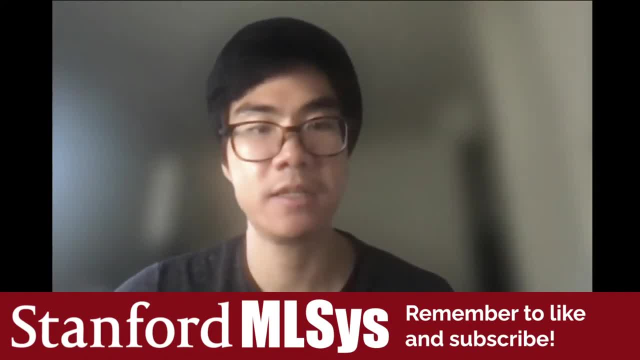 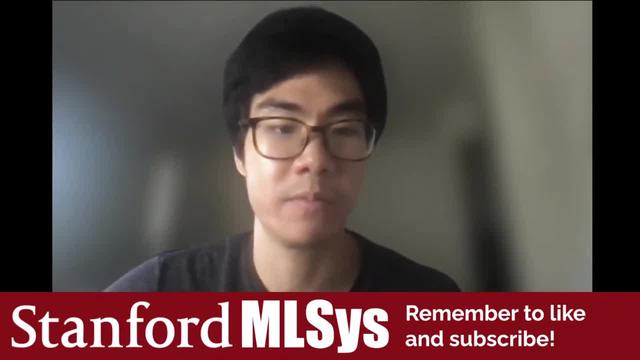 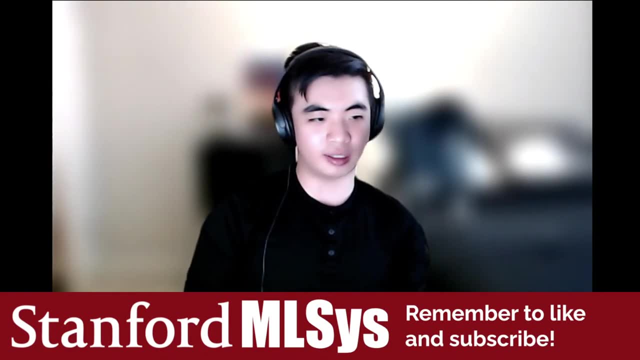 I think there's certainly lots of other ways to try to go about addressing that problem. Albert, I just saw a question in chat which got me thinking a little bit. So Chuck in chat was wondering: have you tried to use algorithms like EM, like expectation maximization, to try to learn the A, B and C? 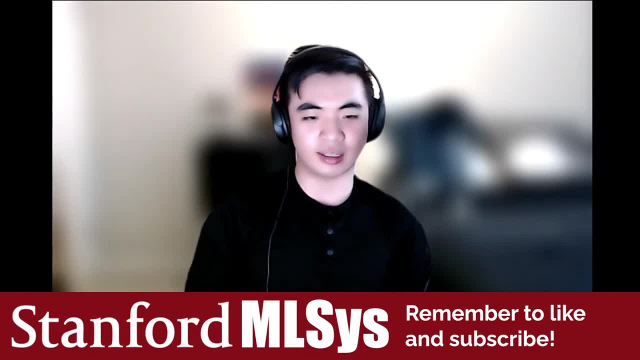 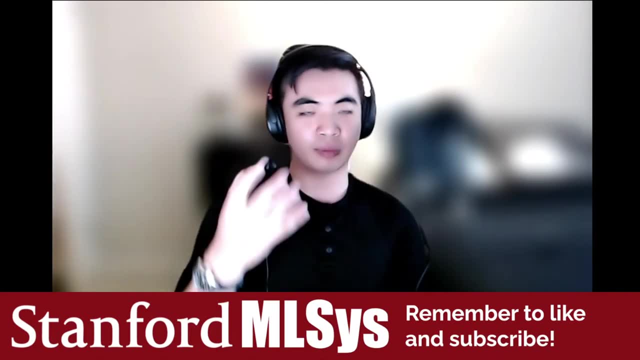 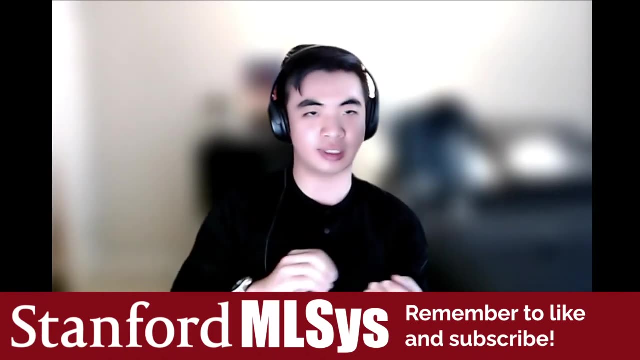 And that kind of got me thinking more broadly. So to kind of in I think the the HIPPO work you you talked about how you derived families of these matrices kind of from first principles, I'm wondering: do you think there are ways that you could arrive at similar matrices or the same set of matrices through some learned approach? 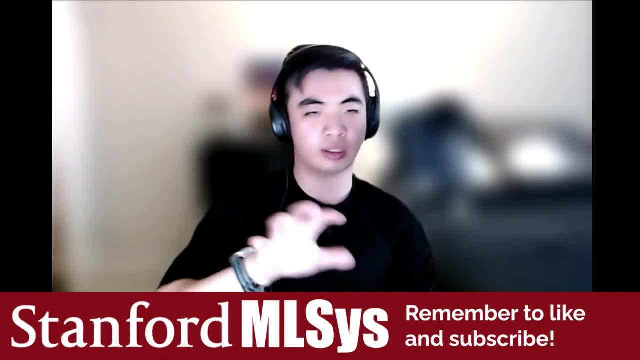 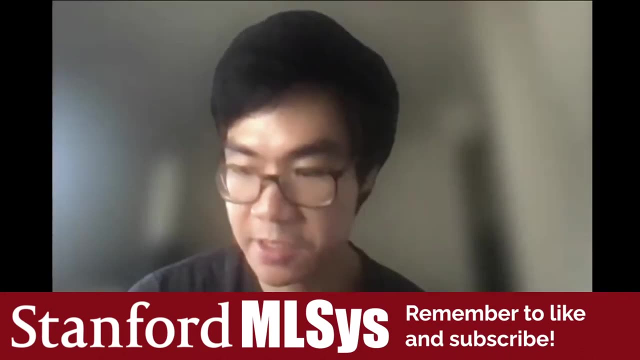 Or is there more, more room in this space to kind of learn what those matrices are And is there a way to train it to do memorization or train it to do But Some other property that we might find useful? Interesting question, Yeah, so. 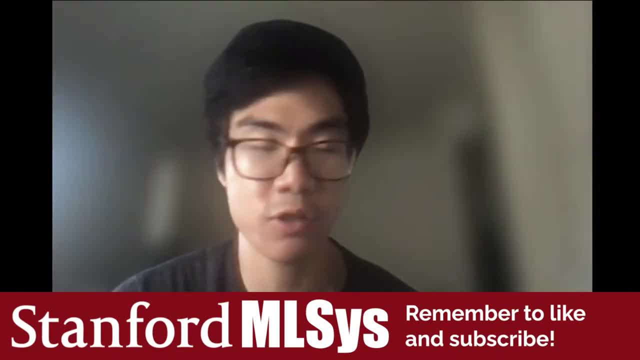 I think so. I guess also another connection. the EM thing also made me remind me of something I didn't talk about much, which is that, as I said, state spaces are Widely used in some other fields, But not so much in deep learning and in. I do know that other uses of it often involve like 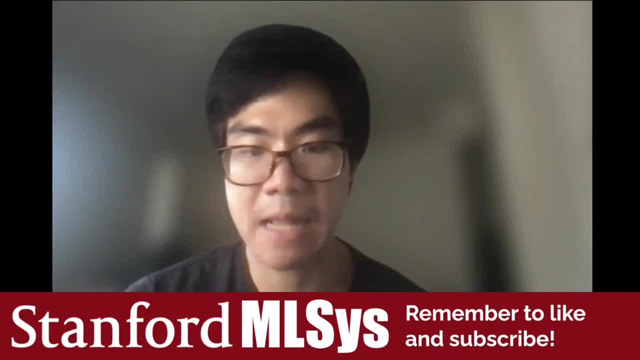 A little more constrained settings where instead of a black box representation you kind of, or you have more specific like input outputs and you're trying to infer the states and then you might rely on some latent variable methods like EM or other things. I view that the application of S4 as kind of a 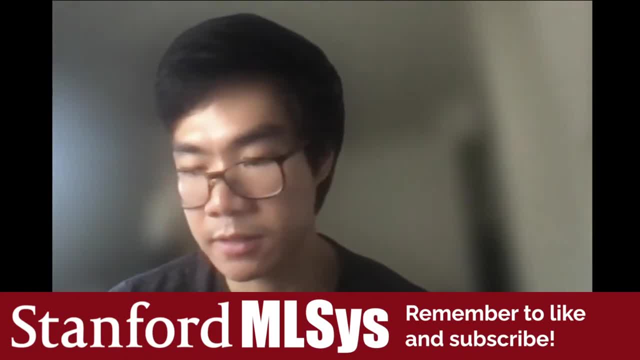 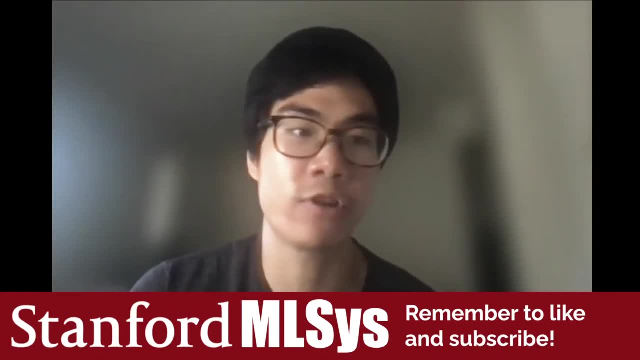 Different, A different use of the model, entirely like when we use in deep learning. we so so far, the only thing we've tried is basically just learning these using gradient descent, And then we've tried using some of the other algorithms that we've used in deep learning. where we have these, 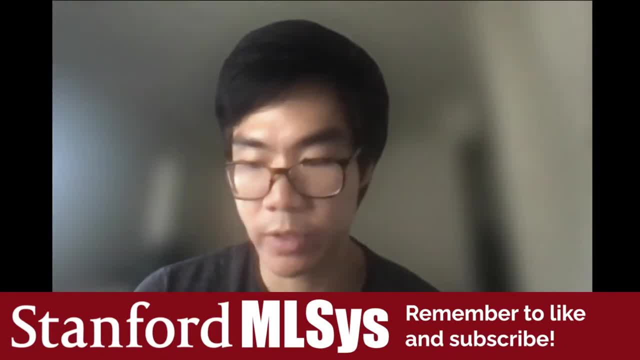 Black box parameters, ABCD, that are learned. We have not tried using other algorithms for learning them. This question is interesting, though, because I did. this does bring up something which I didn't- we actually didn't consider, which is, instead of deriving those matrices theoretically, are there alternative ways that you can derive them? 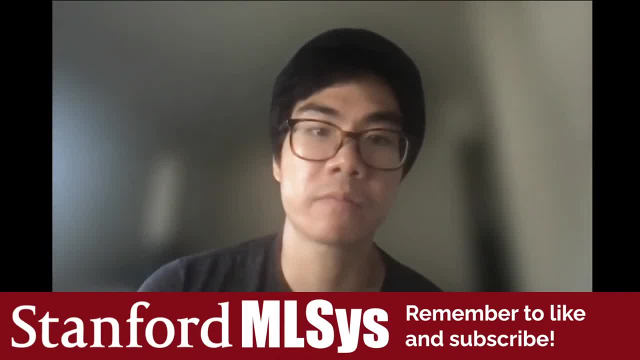 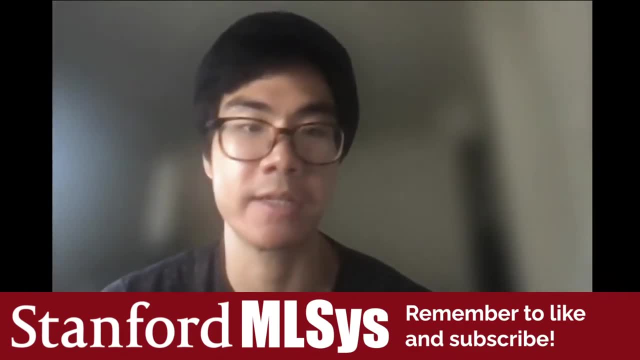 Maybe like empirically, because really, At the end of the day, if you're trying to memorize, You're trying to memorize Something. then what really matters is really like empirically- is it memorizing it or not? And so that it seems like it seems actually quite sensible to try to do something along the lines of what this question is asking. 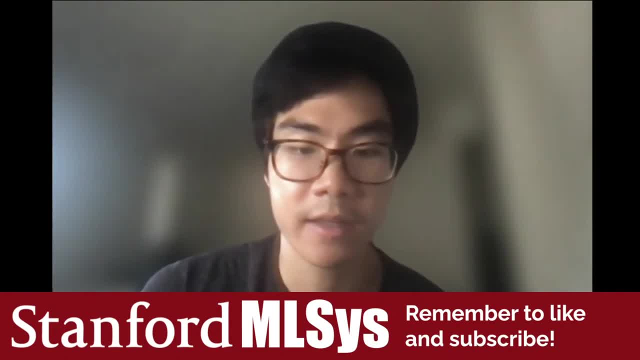 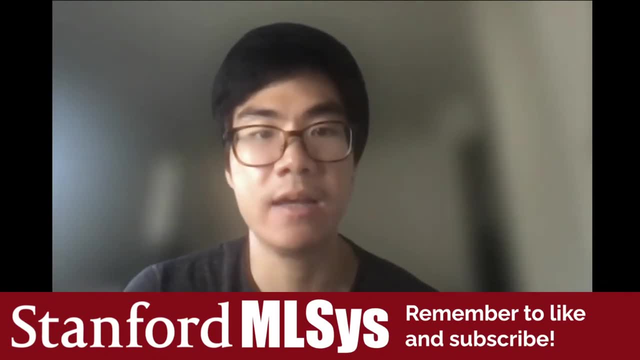 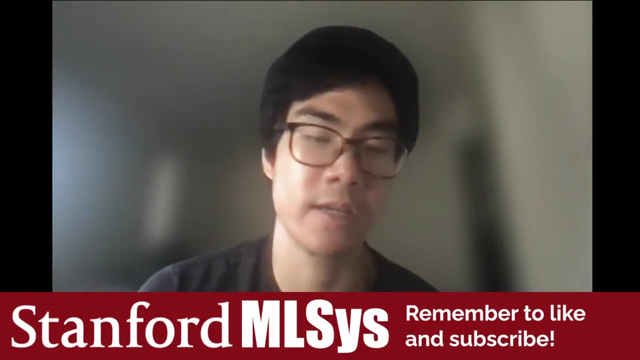 I think perhaps just like trying to learn a very basic state space by, you know, feeding it into output pairs where the sort of in an auto encoding style, where you're trying to help us, trying to reconstruct the input at every point, Maybe you just kind of like the same problem set up as hippo, but instead of doing it theoretically, giving it synthetic data to try to reconstruct things and then using brain descent or EM or any other algorithm to learn the best ABCD matrices. 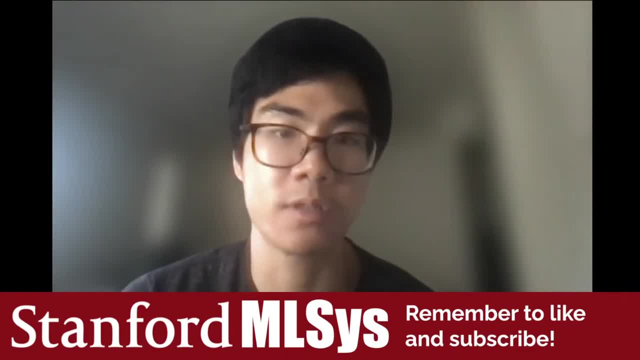 And then that can then potentially be fed in like just use verbatim or just use directly in in the model. So that's something we have not considered at all, but I think it could quite potentially be useful. So that's something we have not considered at all, but I think it could quite potentially be useful. 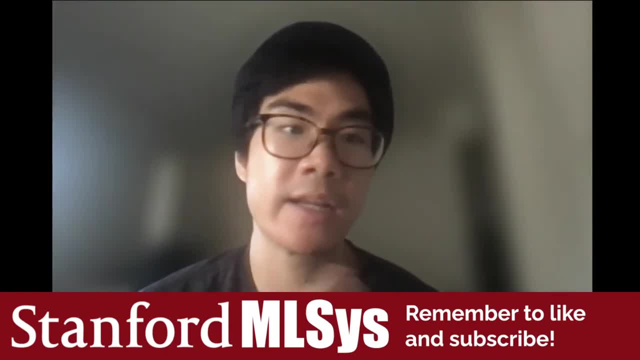 So that's something we have not considered at all, but I think it could quite potentially be useful, especially with some of the connecting back to the previous questions. there might be some alternatives to hippo or extensions of the hippo that involve different bases or other more complicated setups that might be too difficult to theoretically derive. 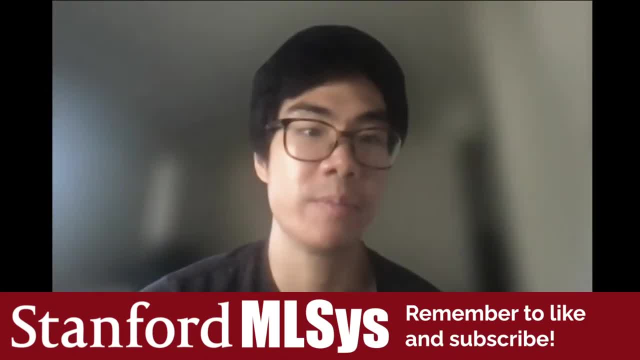 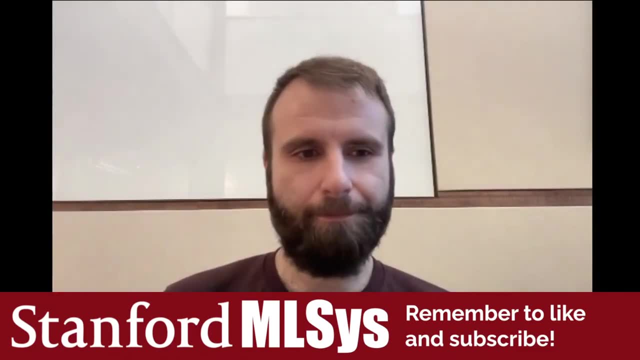 But perhaps you can actually still learn them empirically and do well. empirically interested in If if people are interested in this, please feel free to contact us. If if people are interested in this, please feel free to contact us. We are working on many extensions. 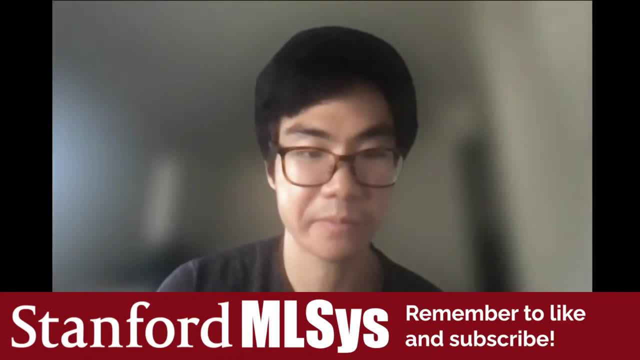 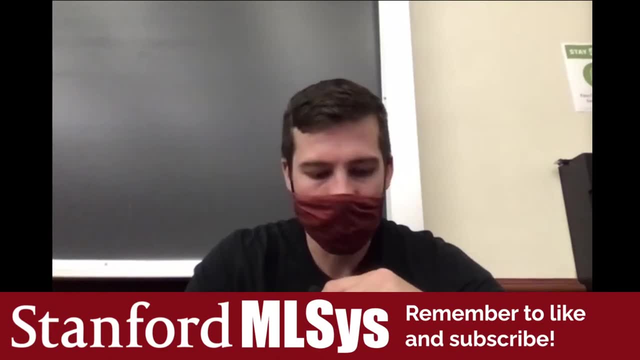 if if people are interested in this, please feel free to contact us. We are working on many extensions. Great Albert, I was wondering if maybe you could provide some, you know, higher level intuition about what s for does, better than these other sequence models when it comes to like learning. 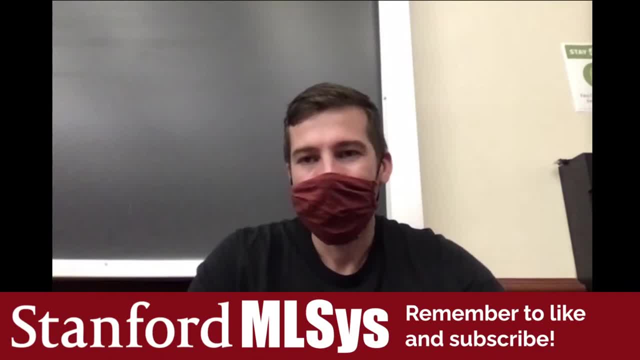 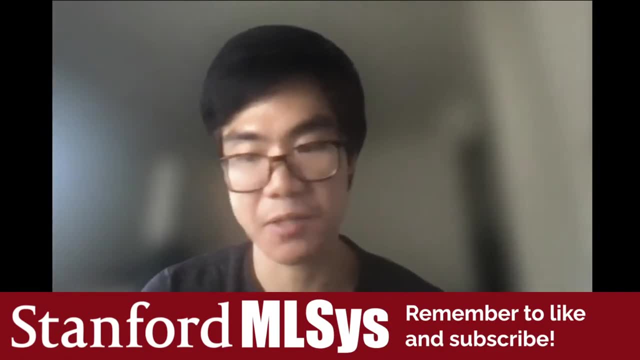 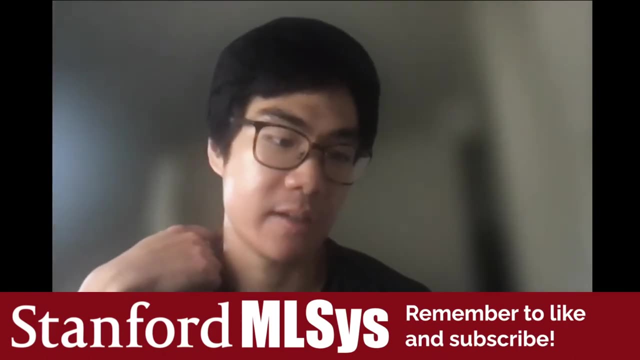 What is it All right, okay, Great, Thank you. I guess it's a bit hard to define what learning more complex things means Certainly like the way it's constructed. it is constructed to not forget things, So I think that the types of data where it would do best on are sort of like sequences. 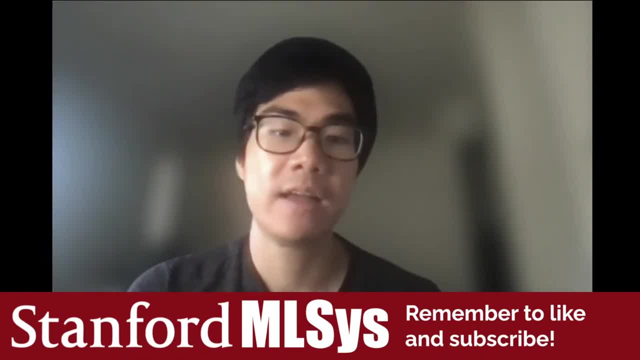 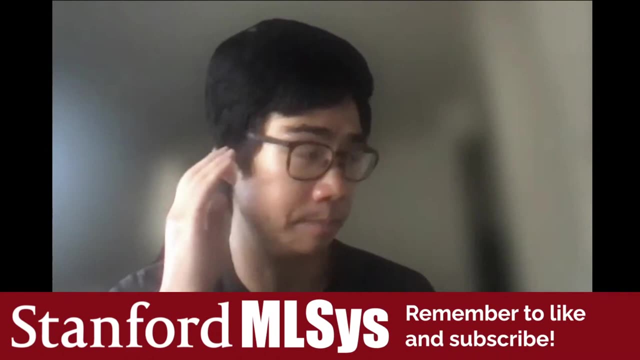 where you need to be constantly like looking back and you need information about a lot of context at every single time step, if you're making a prediction every time step or doing something and you just need lots of context. I think that's where S4 particularly excels at. 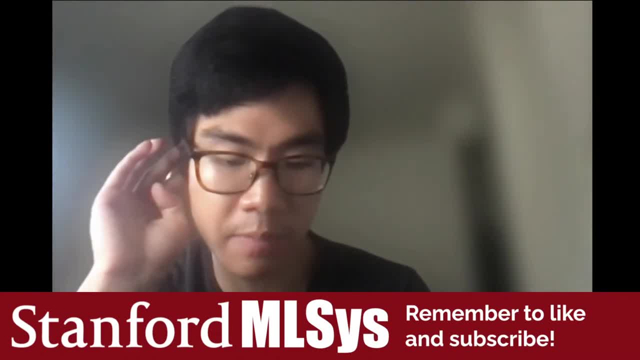 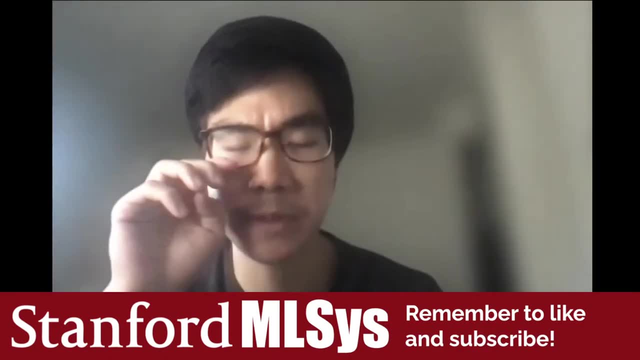 There's a bunch of other. So, compared to other sequence models, there's a bunch of other properties that S4 has. I think that makes it attractive because of its multiple representations and some of these were hinted at in the presentation- Because it's continuous. 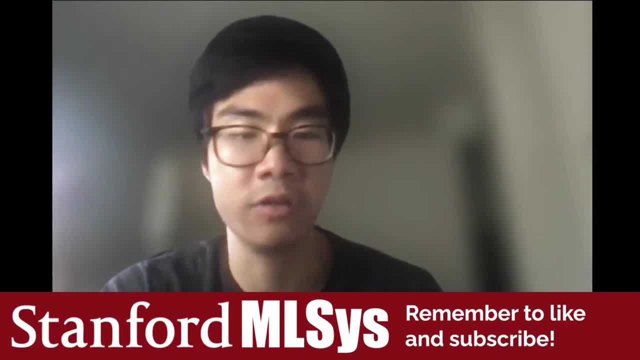 It really. It really seems to do better at continuous data than other models. So for the examples I gave in the beginning with the ECG, EEG data and speech and so on, those seem like particular domains where S4, compared to the baselines we've seen- S4 seems. 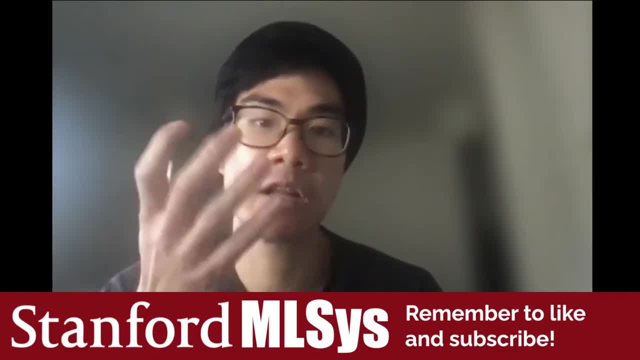 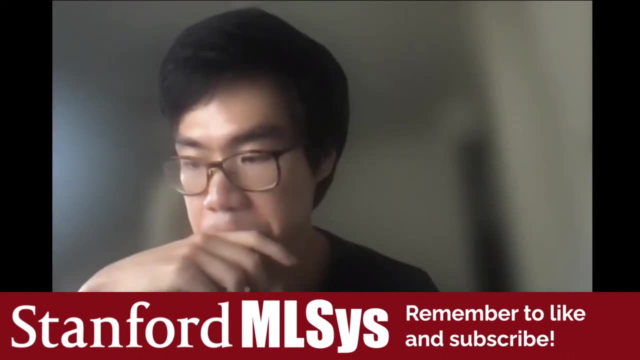 to have a lot of promise at doing better there, because it's modeling a continuous process and it's using this theory that allows it to capture a lot of context. Yeah, there are other properties that make it nice. There might be kind of more on the computational aspect. 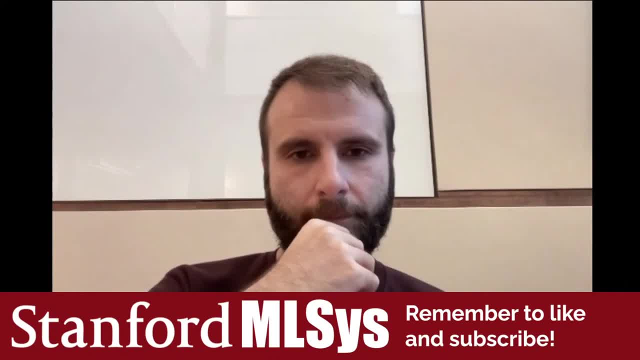 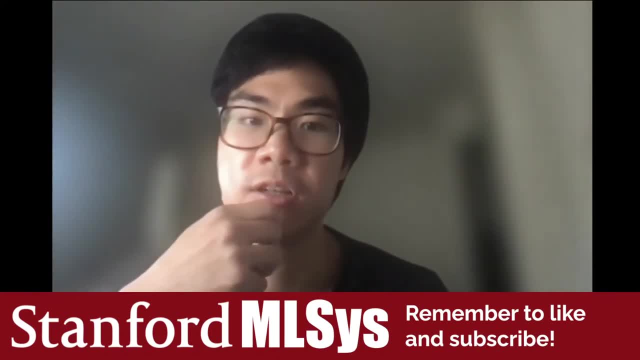 I don't know if, Yeah, I mean it's not like a free lunch, It's not just going to be better than everything else, but it has been generally good on most things. we've seen There might be some trade-offs compared to other models. 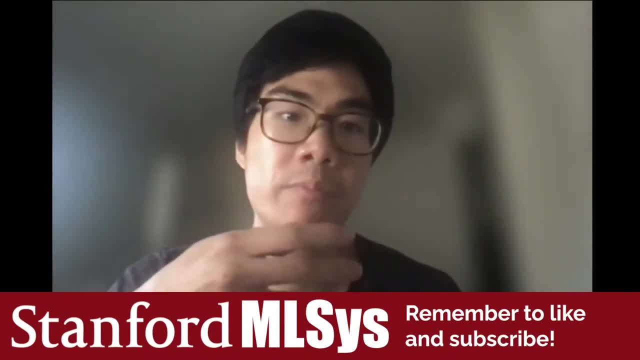 Like I mentioned, on discrete data or in shorter data, perhaps transformers are better. There might be- Yeah, Yeah, There might be- some types of data where CNNs are more efficient, at least perhaps also do better. In terms of what we've observed empirically we have seen S4 generally seems competitive. 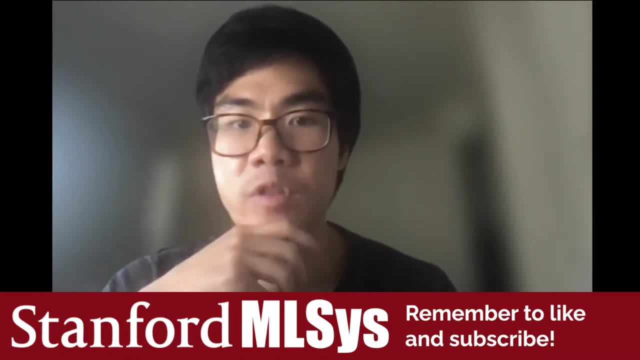 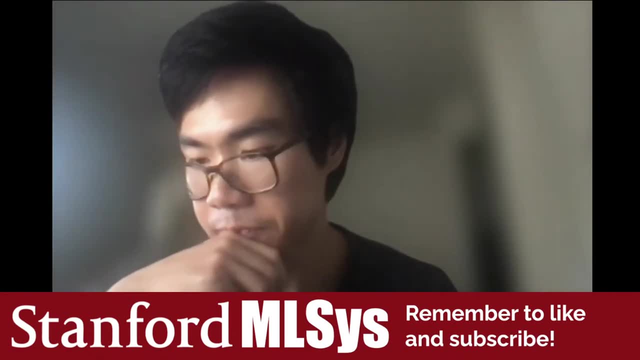 with RNNs and CNNs across the board. There are areas where transformers seem to be doing better right now, but S4 is still pretty good. But yeah, in terms of the actual where it excels, it really just comes down to the theory. 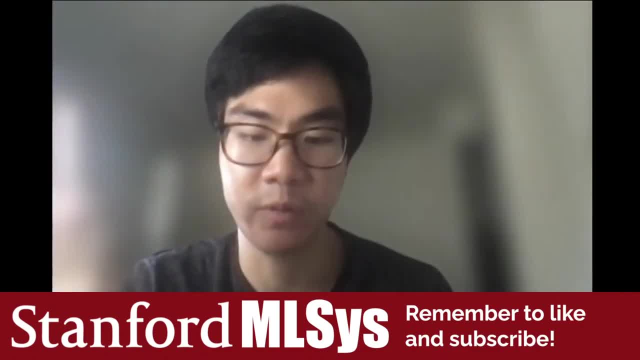 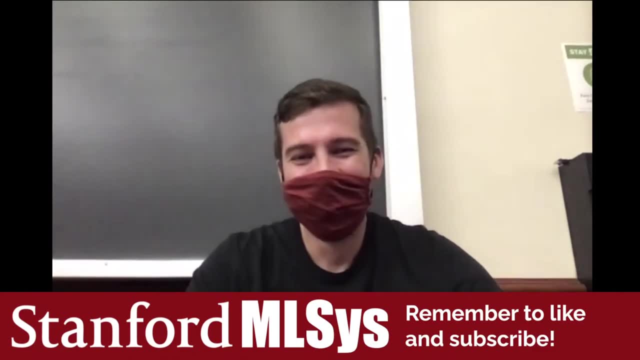 It's a continuous model, it's good on continuous data and it's good when you need a lot of context. Perfect, That's exactly the kind of answer I was looking for. Thanks, I think, Albert, you could also potentially test some of this hypothesis to a certain. 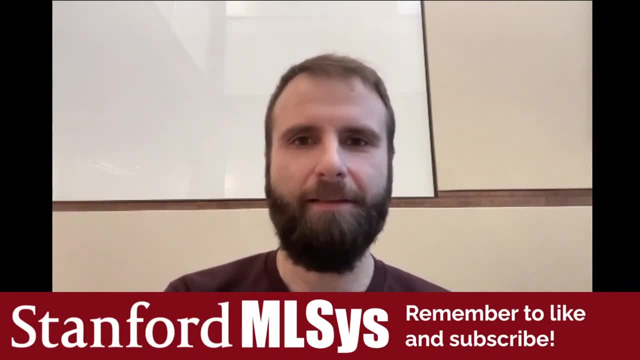 extent right. You could create some synthetic data sets that maybe you can test for how long the dependency, For how long you can remember something right, Or for how many things can you remember after a certain amount of time, Or for how complex in terms of the power of the polynomial, for instance, something 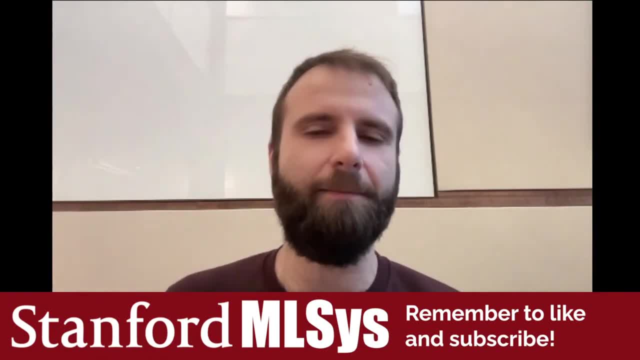 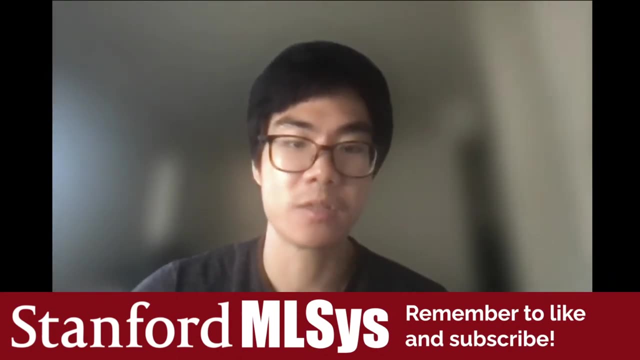 that you generated at the beginning is then being able to be reproduced later on. So I think you could have a way to quantify that to a certain extent, right? Yeah, that's a great idea. I think we considered incorporating some of these on our most recent paper as well. 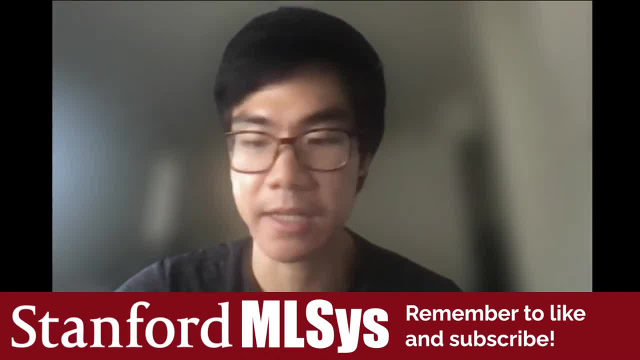 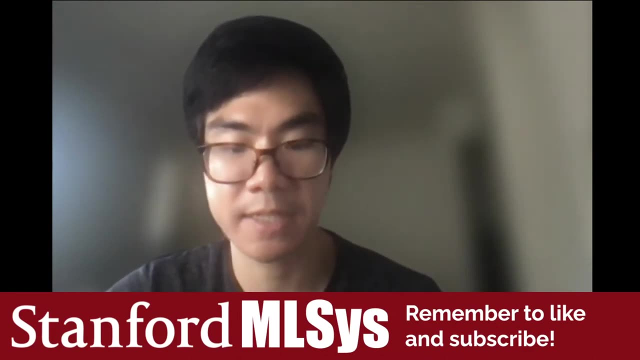 We ended up, not for space reasons and time reasons, I guess, But we are actually still interested in kind of a more controlled evaluation of how much it can memorize and what dependencies it can handle compared to other models On the preliminary things we've seen. it does, I think, do as it claims and really handles. 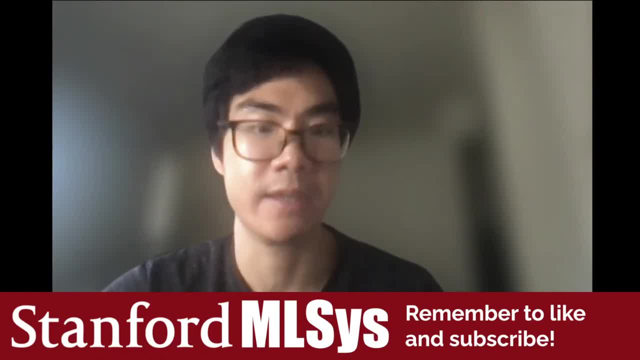 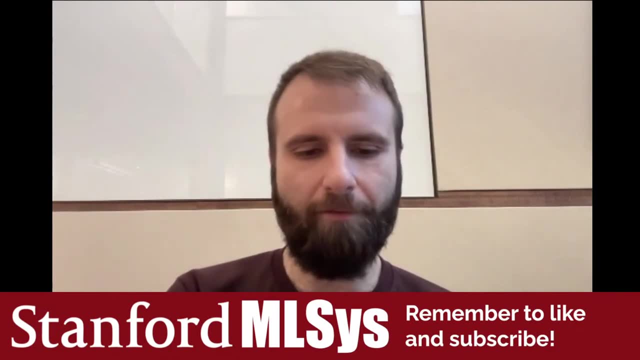 these long things well, But certainly a more controlled setting, I think, would be a nice comparison point at some point. Yeah, I think just to do one little step back on one thing that we touched upon before, like you know, Basically, the creation of these matrices A, B and C, in particular A, you know kind. 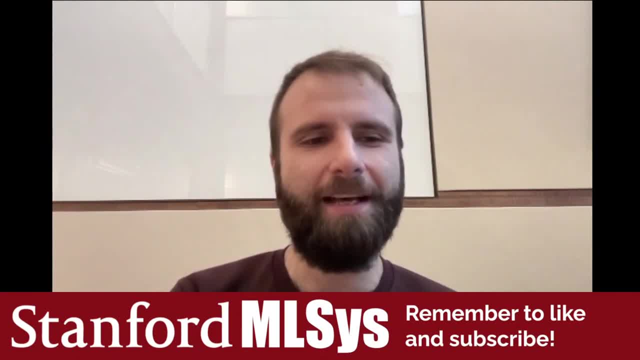 of biases, if you want the model towards memorization right, And the hypothesis of potentially learning these matrices through other mechanisms makes me think of potentially, I don't know- something that sounds like a curriculum to me, something that sounds like: first you learn to memorize something and then the model learns to exploit. 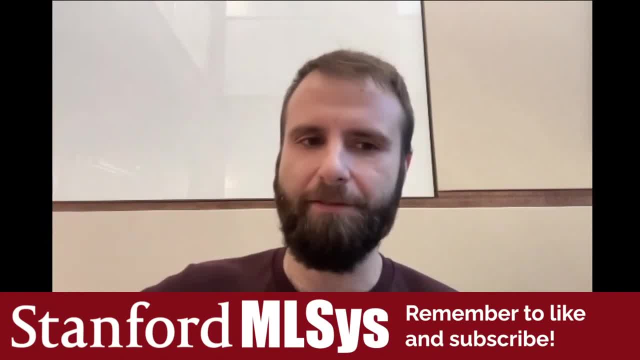 this capability of memorizing for learning to do some other things right? Is it like anything? that is like: have you thought about that or does it make sense to you? I'm curious. Is this like a direction? interesting thing to think about. 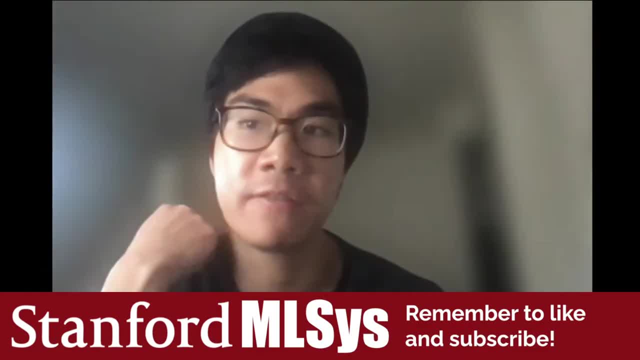 So that's actually related sort of to our original motivation for designing the model, where I mentioned that the model kind of came about from Hippo first, where we first, we first, We first had this Hippo theory which gave you this A matrix. 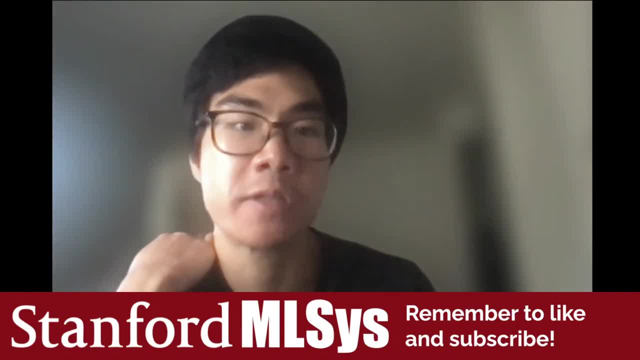 And then we're trying to figure out how to exploit it, Like how do you actually use the thing you've memorized? And that's where the idea for projecting it using these C and B matrices came from. So it's not- It's not exactly answering your question about curriculum, but it's kind of like motivation-wise. 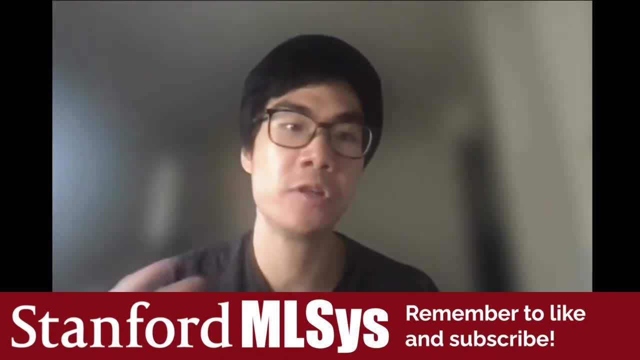 that is actually how we were thinking about it. We wanted to design a model that first has a mechanism for memorizing and then has some additional mechanism for exploiting what it's memorized And that naturally separates into the first equation, which is the A and B, with the Hippo. 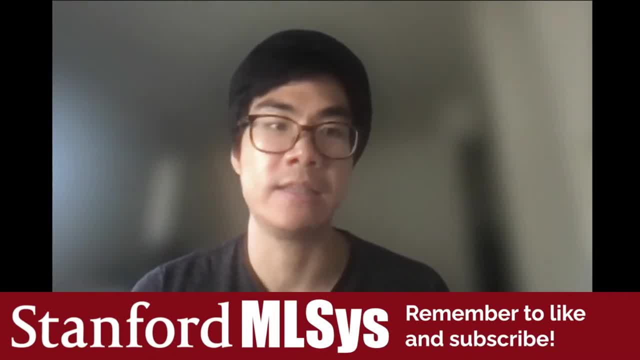 and the state, and the second equation, the C and D, that uses the information it's memorized And that, like I mentioned, the A and B are actually initialized to the exact formulas given by the theory, whereas C and D are kind of more generic deep learning parameters that 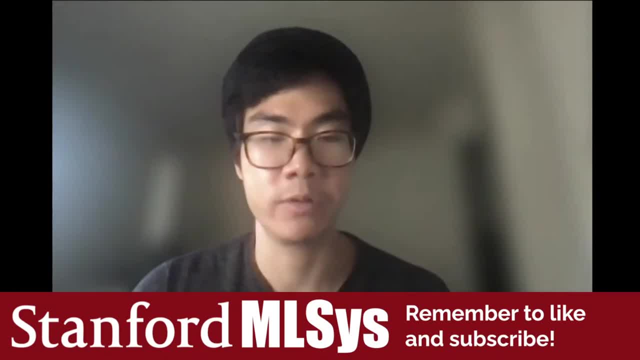 are initialized randomly and then you just learn the right way to exploit it. That makes a lot of sense. Yeah, Thank you. Thanks. Your question about curriculum also reminds me of some other applications that we've thought of, that kind of like pie-in-the-sky applications that might be interesting but related to 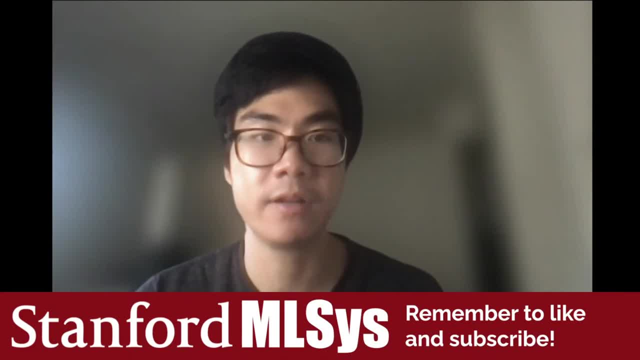 what I mentioned about how it can work on sequences of different sampling rates or resolutions. we were wondering if perhaps you can do something where you first like train on shorter sequences by subsampling it and then gradually make your sequences harder and longer, and like 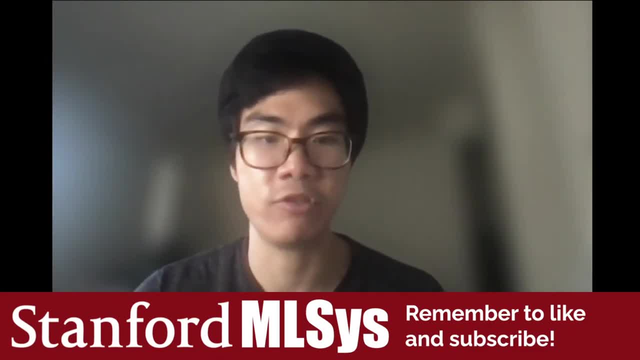 fine-tuning the information, Using like the higher resolution information in the data. That was just another random direction we had thought of before. That is super interesting. I encourage you to also try that out. I'm super curious to see if it actually helps. 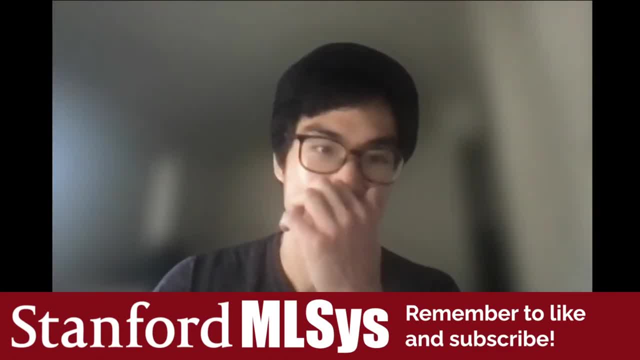 Yeah, Albert, as we kind of, I think, get to the end of the hour, I wanted to give you a chance to kind of talk about what is in the future for you and your research. What can we expect in the next weeks, months, potentially years, as you start working on? 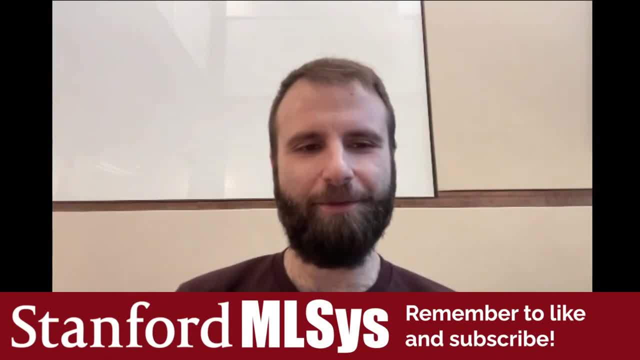 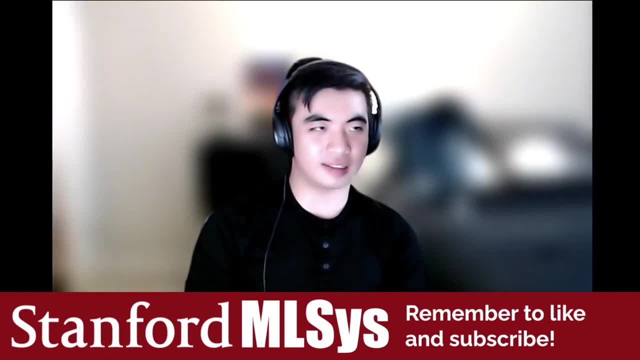 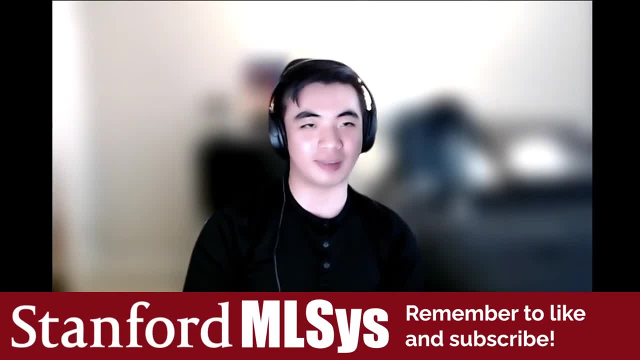 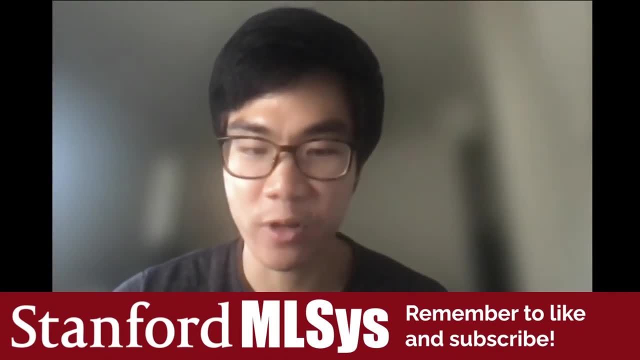 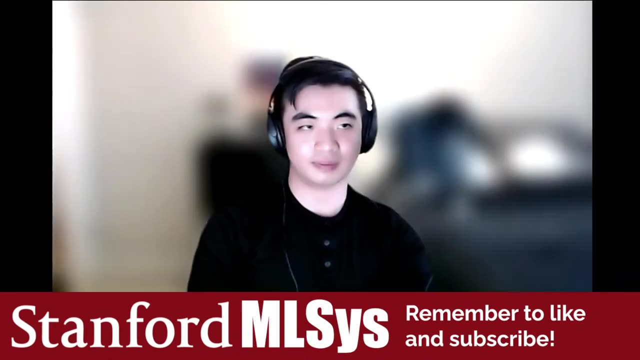 independent research. what is the next line of work from the great Albert Gou? Well, I think a lot of the short medium term work I'm interested in are going to be built around this, As we've kind of touched on many different applications and extensions of it already. 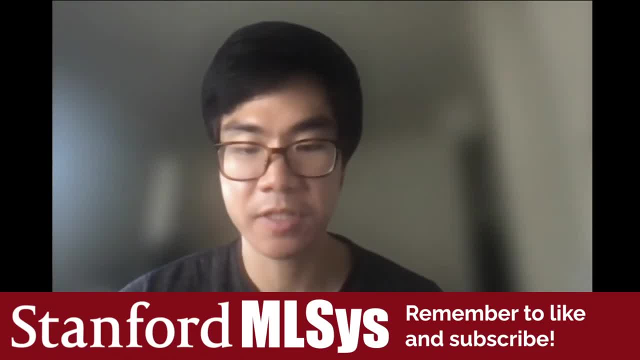 in this discussion. there's just so many. I think there's so much potential for using this. as for more applications of this model and extensions of the ideas, On the theory side, there's all of these questions about: like the question about: can you generalize the theory? 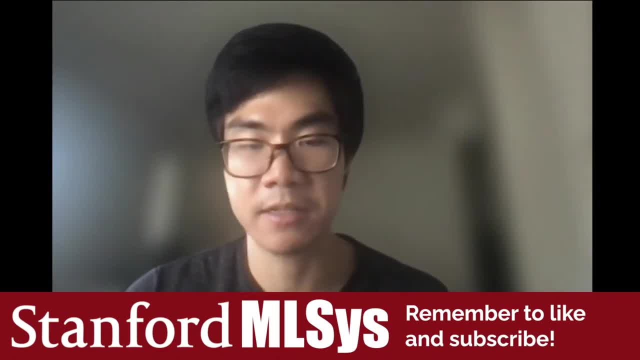 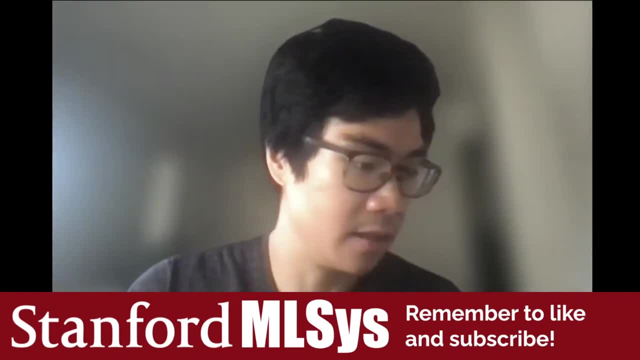 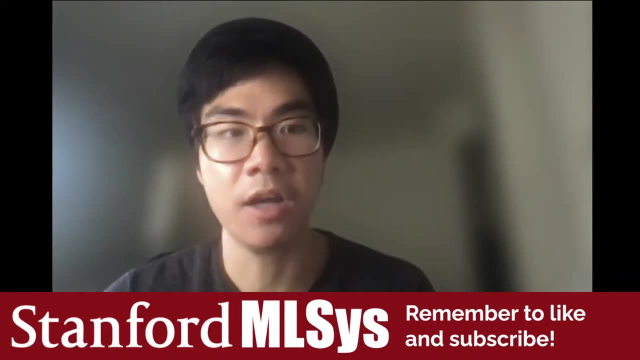 and use different bases. Something I mentioned is: can you generalize it to higher dimensions? And that naturally opens up a bunch of applications. In terms of applications, there's all the you know, there's different data modalities, There's all this like long document text stuff. 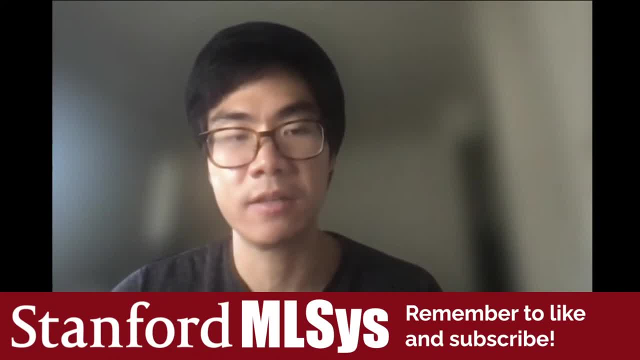 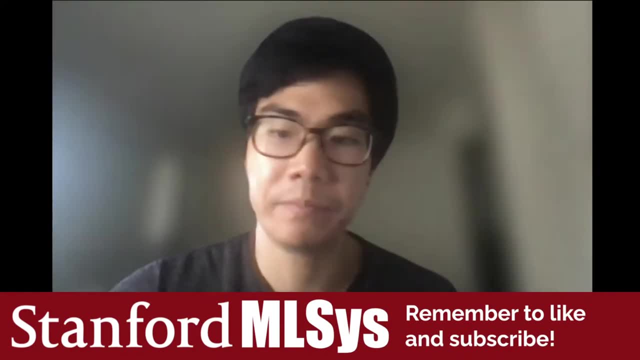 There's we're interested in, like larger scale audio or ECG data, So there's a lot of promise there, I think. higher level. I'm really interested in how to continue designing models that can handle at larger and larger scales, that can handle more and more context. 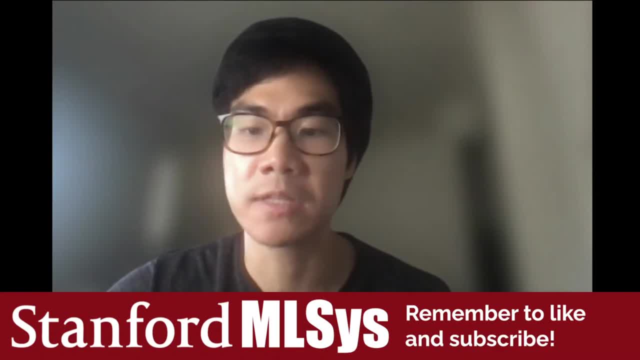 Eventually, it would be really interesting to have you know models that can generically synthesize I don't know like sequences that are millions of times steps long, If you really, if you want to do like an entire, like speech or something, 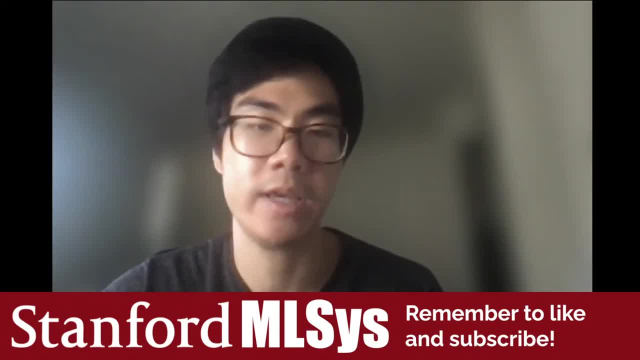 And to do this kind of in a generic deep learning way without substantial, you know, architecture engineering or future engineering, engineering, stuff like that. There's lots of technical challenges that come with this, like the theory side of how do you memorize. 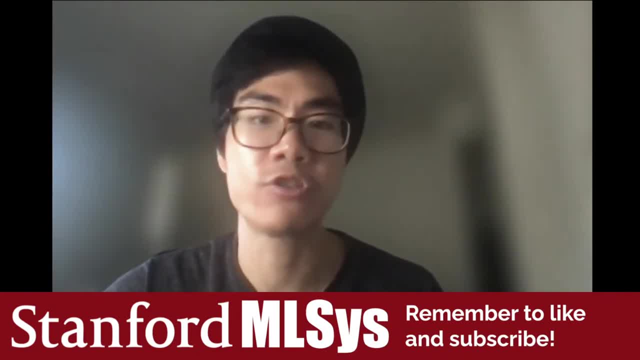 but how do you like, how do you actually train on something this big You can't like when you can't fit this thing in memory? So both on the modeling side and on like computation or engineering side, there's lots of challenges there. 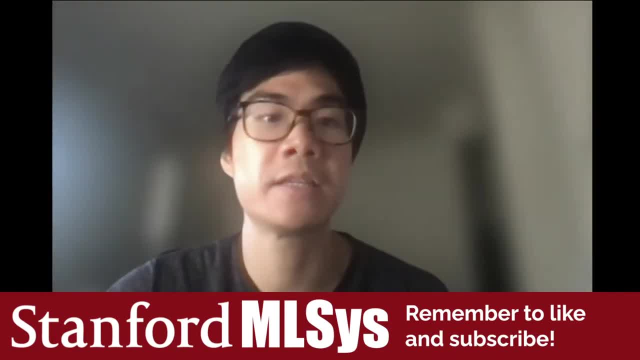 It does seem to me like, eventually, this is something that the field has to move toward anyways, because we can't keep using fixed context models forever for a while, as we get to more complicated tasks and more and more data, um. so i think that models such as this 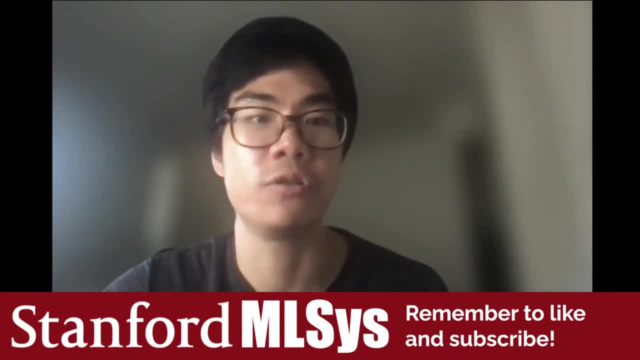 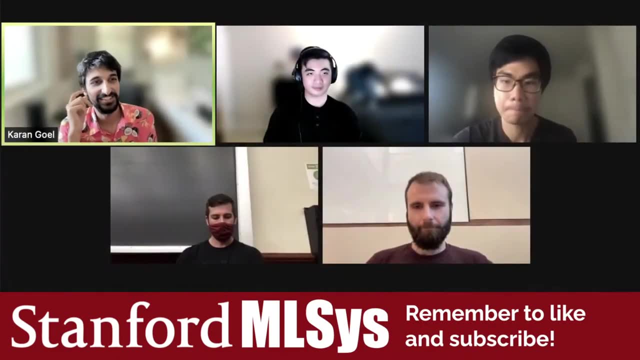 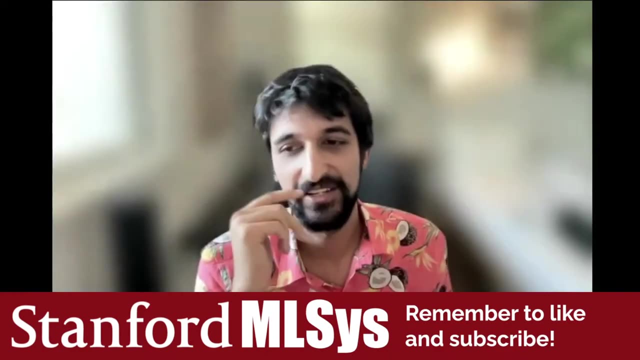 are definitely one really have a lot of potential for moving toward that direction. awesome, i, i think we have a couple minutes. i just want to sneak one last question in which maybe is a little bit philosophical, but like, um, i think one thing that i'm curious about is 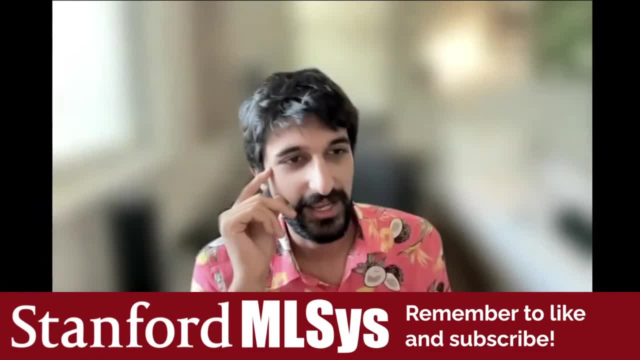 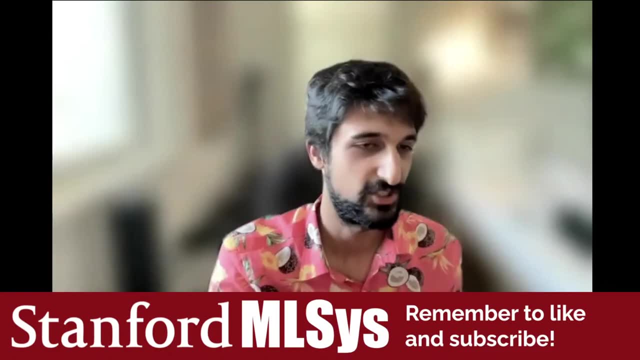 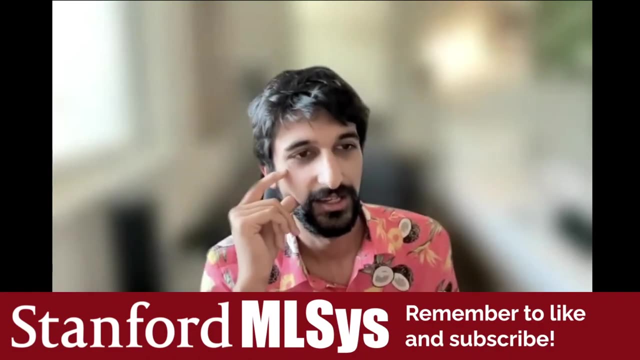 you know you, you've been studying kind of memorization um as a problem, and you know different tasks. we generally with s4 train different models for those different tasks. right, and generally in machine learning as well. like you have people who train you know transformers for text, or you train convolutional models for, uh, image data. uh, i'm curious, you know memorization. 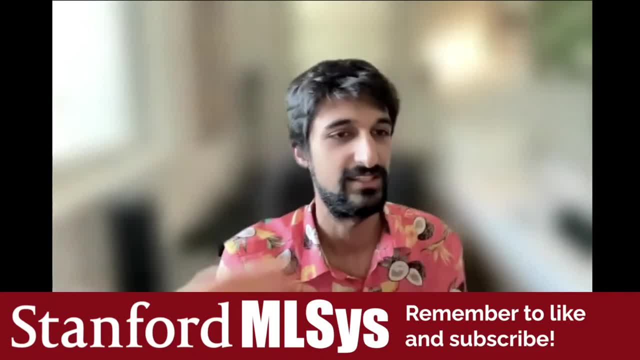 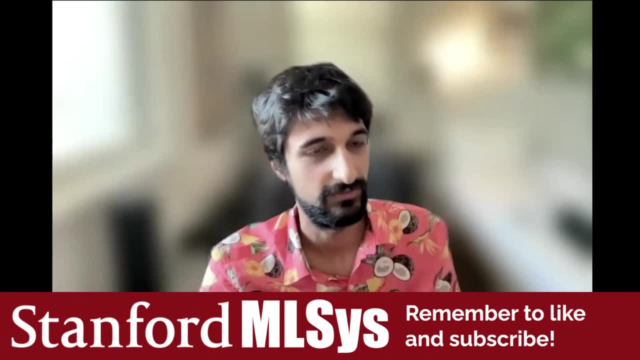 as a skill, even in humans, is kind of you know it's the same skill but you apply it to many different domains. right, like you remember things in math, you remember things in language. so it seems like it's kind of independent of the type of data that you have to deal with. so i'm curious if you've thought 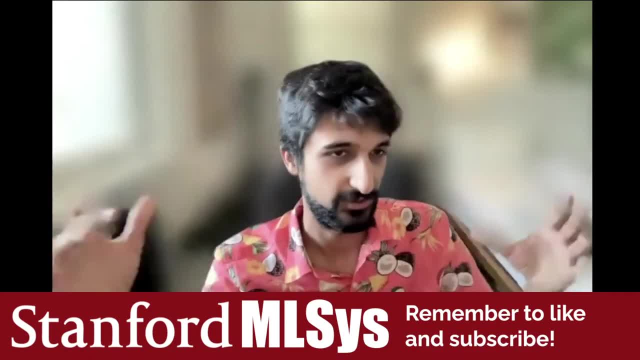 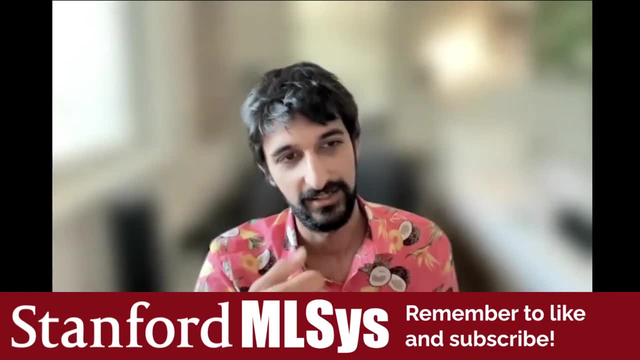 about. you know how one could bring that all together. you know training on all these different modalities and and sharing this, this core skill of being able to memorize long sequences of data um across them. yeah, i mean, i think one way of looking at it is sort of like: